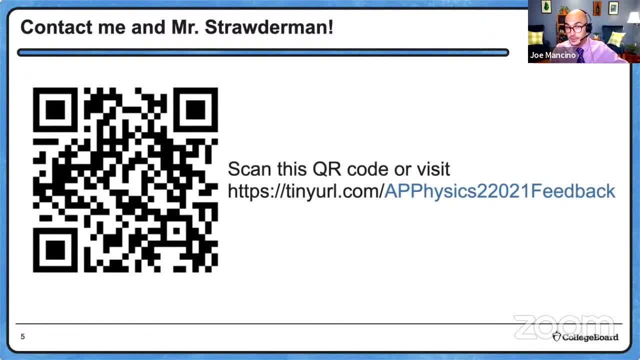 you should take a look at this QR code. Take a look at that tiny URL. That's tinyurlcom. AP Physics 2, 2021- feedback. I really appreciate the feedback that I've been getting and I would. I hope Mr Strauderman takes all your feedback and works it into tomorrow's session. So thanks. 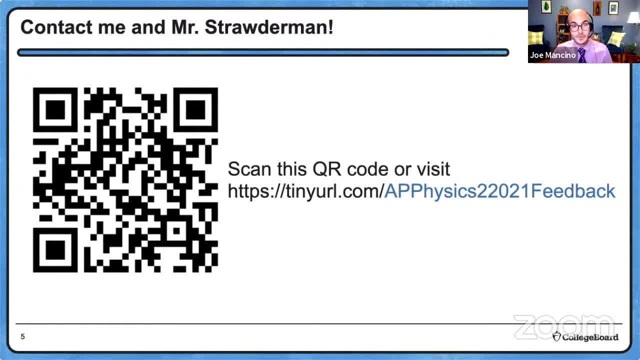 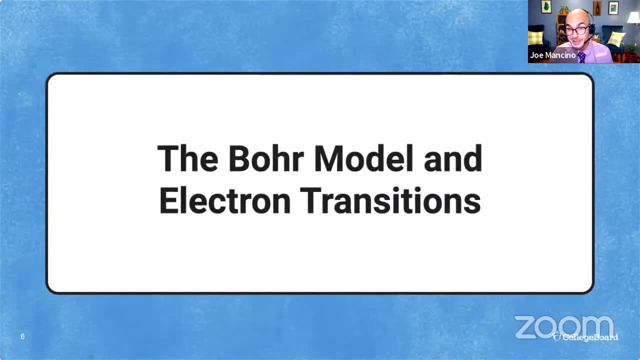 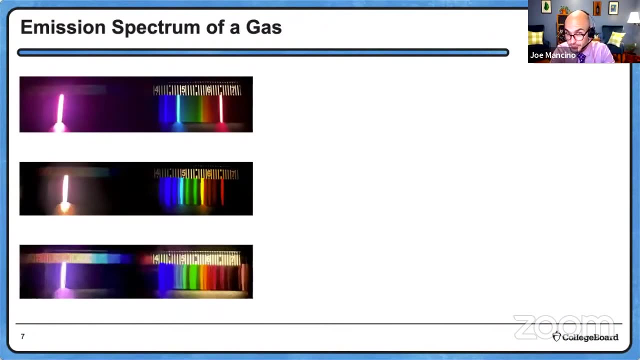 to all of you. Thank you very much. We will be discussing that toward the end of this presentation. So thanks a bunch. All right, We're here to talk about, first off, the Bohr model and electron transitions. Now these photos show the evidence that we have for the Bohr model, The modern picture of the atom. 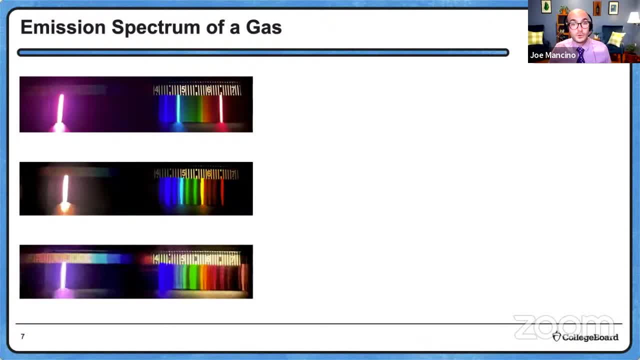 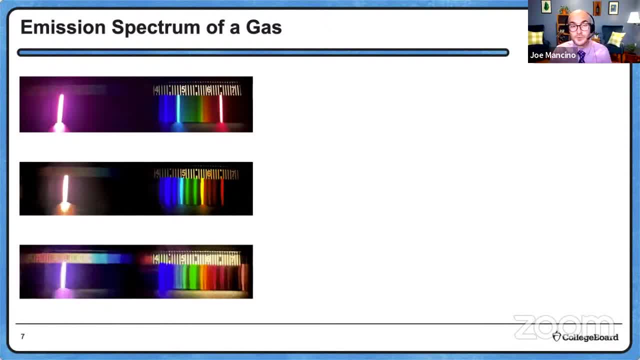 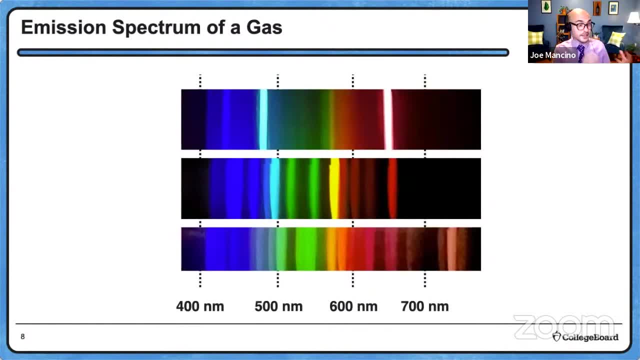 grating, we get the spectra on the right side. Now, those rainbows of colors, those spreads, uh, they give us evidence that classical physics could not explain. We needed to refine our ideas, uh, about atom to uh atoms to explain this evidence. So, based on the observations that 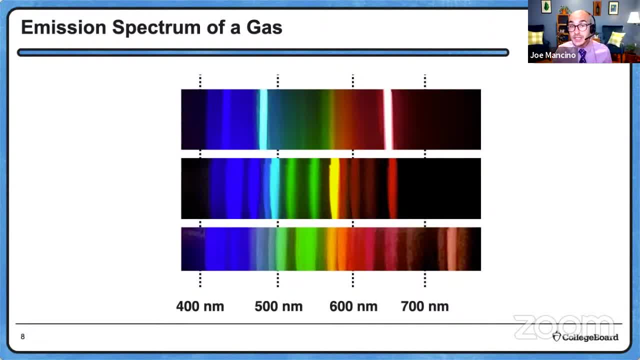 scientists made, the mathematical work they done and the leaps of reasoning that generations of scientists did, we've painted a much newer and more nuanced picture of the atom. So let me take you through some of the things in what's called the Bohr model of the atom. Some important features: 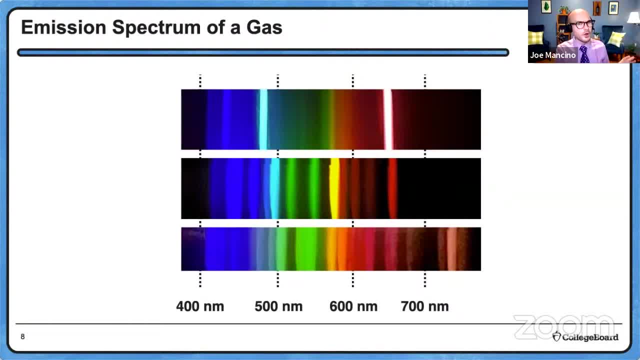 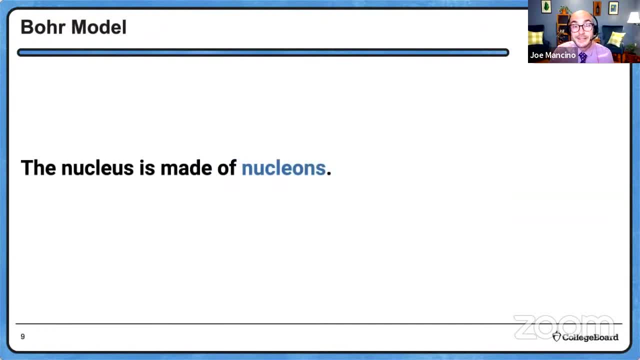 of the Bohr model of the atom. The Bohr model of the atom is a more modern uh view of the atom, although not the most current model that we have today. In our model of the atom, of course, the nucleus is made of nucleons, which includes neutrons and protons. The nucleus is surrounded by 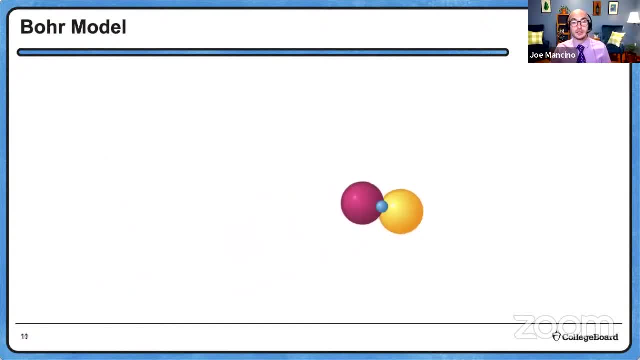 electrons right there. Oh, look an electron. Uh. historically this Bohr model has been used to represent atoms And in this model electrons circle the nucleus like planets circling a star. In this model it would be the electrostatic attraction between electrons and nuclei that hold the nucleus. 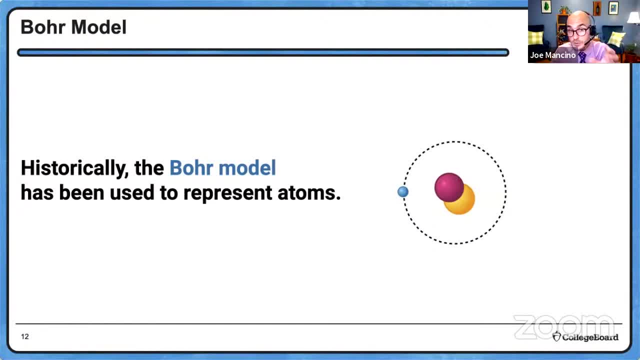 together. It's not perfect. It's a good model and it makes good predictions. It's practical. The Bohr model works for larger atoms too. You may have used it in your chemistry class previously, uh, to talk about the chemical properties of matter Today. 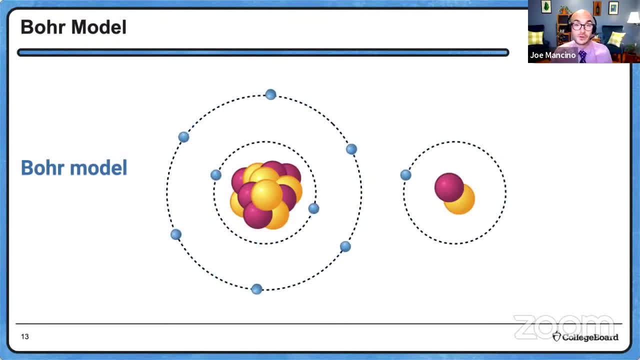 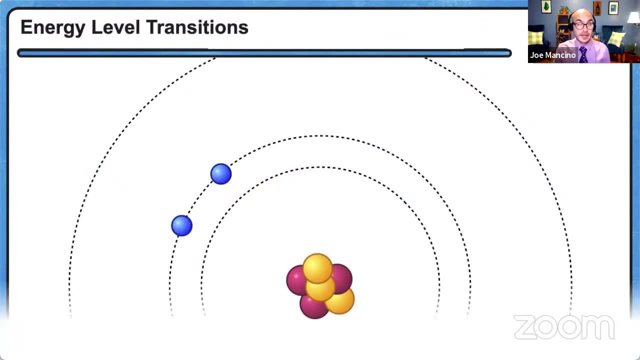 we'll be using it as a really good stand-in for the modern picture of an atom. So the difficulty of classical physics in explaining atoms arose from the fact that atoms can only absorb and emit energy in discrete amounts, That's countable amounts. 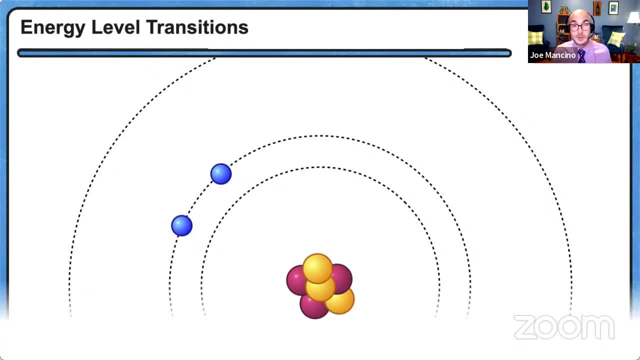 Only very specific amounts that atoms can absorb and emit energy. The specific light energy that the atom's electrons can emit or absorb depends on the organization of the atom itself. This is the case when a few different types of electrons connect with each other, meaning the particles themselves and not the atoms themselves. 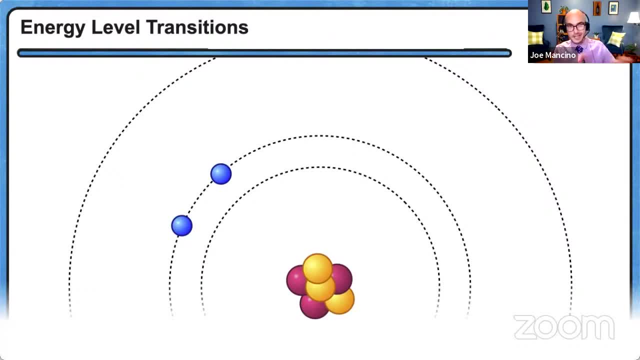 So it's the atom itself that's making the state of an atom. but we can also use electrons in other ways. We can use electrons to make things bigger, or we can use electrons to make things smaller, or to make things smaller or to make things bigger- whatever that we like. 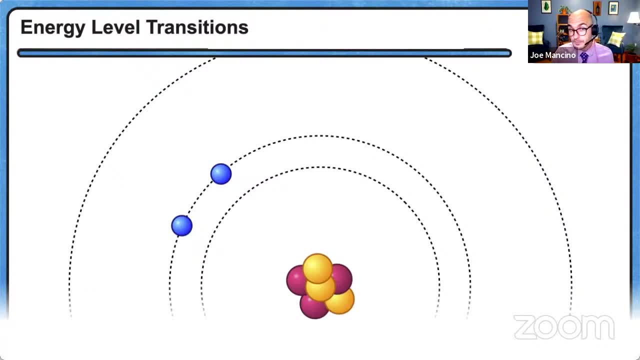 Here are some examples of what's been done here. Let's start with just a small example. all And we need a lot of analogy and metaphor to discuss what atoms are doing. So our modern picture of the atom answers the question: why is it that atoms only emit and absorb light? 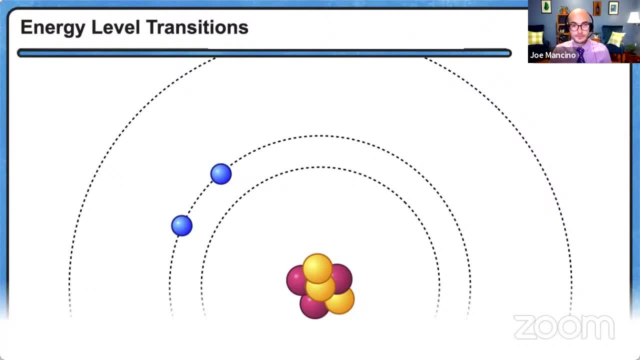 in these very discrete amounts. Well, check out the electron on the right. It's going to emit some light and then change. pardon me, the electron on the left emitted some light and now it's going to change energy levels And you'll notice that it just jumped down an energy level. It didn't. 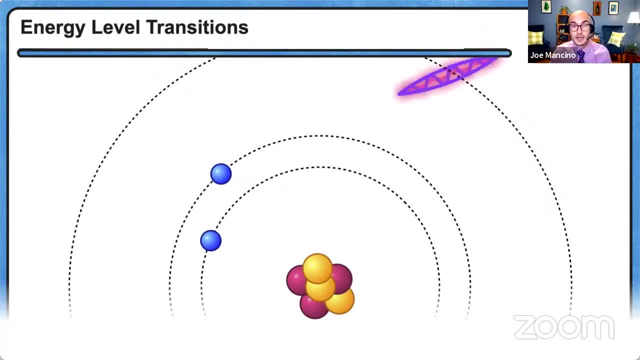 move down. it simply was: The electron on the right had just absorbed a photon of light and it jumped up an energy level. So in both cases, a single electron emitted a single photon of light. In order to tell this story, we need a lot of analogy and metaphor to discuss what atoms are doing. 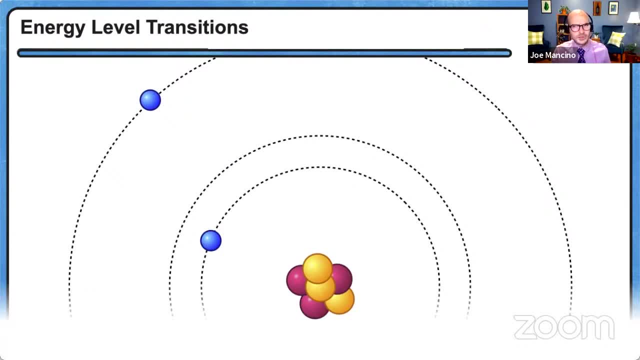 So, in order to tell this story about atoms and what they're up to, and electrons and why they transition, we need to invoke light's particle nature, The idea that light can be emitted in these tiny bundles called quanta, And those tiny bundles of light have energy that depends on their 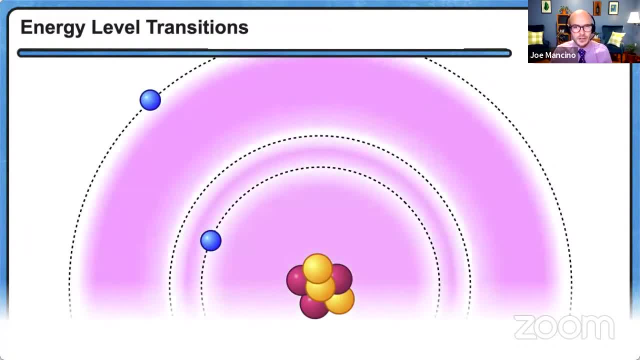 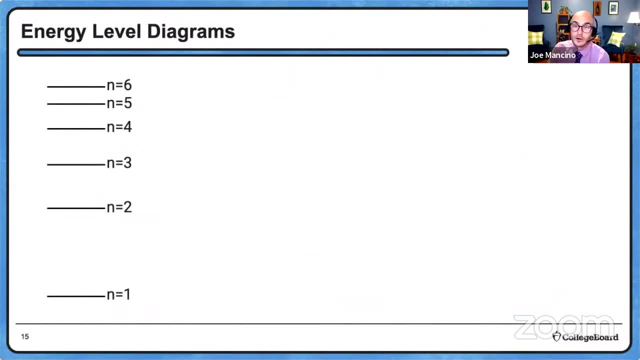 wavelength. In our modern picture of the atom, electrons are never between energy levels. So when I say energy levels, what I'm referring to are very specific disorders, And when I say energy levels, I'm referring to discrete amounts of energy that the electrons can have. And the deal is, the electrons can. 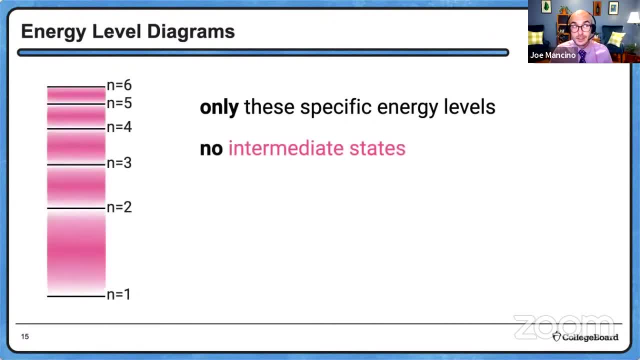 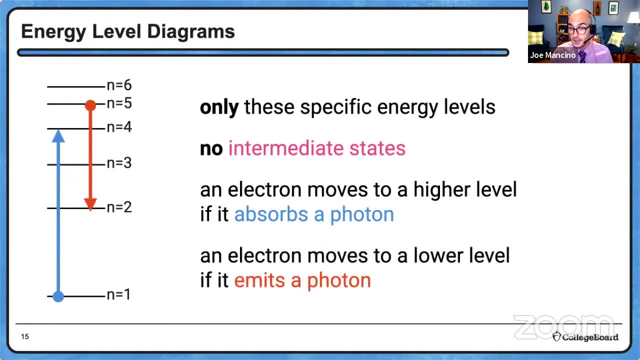 only have those specific energy levels, with no intermediate levels. If an electron moves to a higher level, it absorbs a photon. An electron that absorbs a photon goes up a level. An electron moves to a lower level when it emits a photon. Okay, If you've learned about this in class. 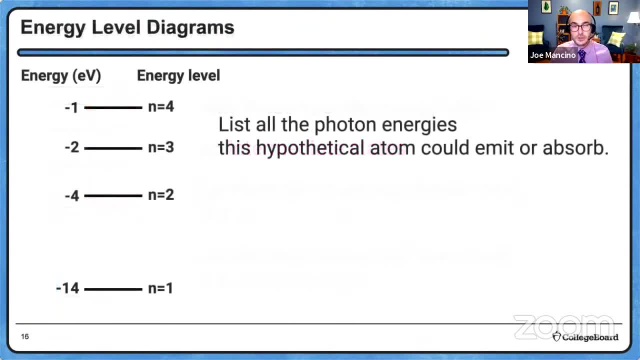 if you watched the AP Daily videos. this next one is going to be easy. Can you list all of the photon energies that this hypothetical atom could absorb or emit? You may want to pause here and count them up. I can wait too. 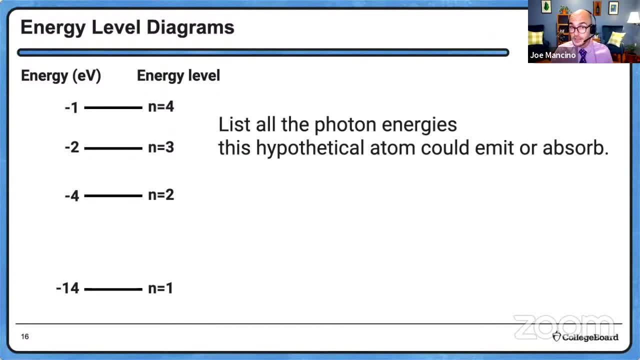 Every possible energy transition would represent an electron moving from one of those four levels to another level And we would know the energy difference based on the difference in electron volts between those levels. All right, Here they are. If you didn't guess all of those, you may want to go back. Pause it, Find out. That represents every possible difference And here's just two. For example, there's the two electron volt level and the 13 electron volt jump. This atom could absorb two EVs worth of energy and jump from the N equals 2 to N equals 3 level. An electron could make that jump. An electron could also jump from the N equals 1 to N equals 4 level. 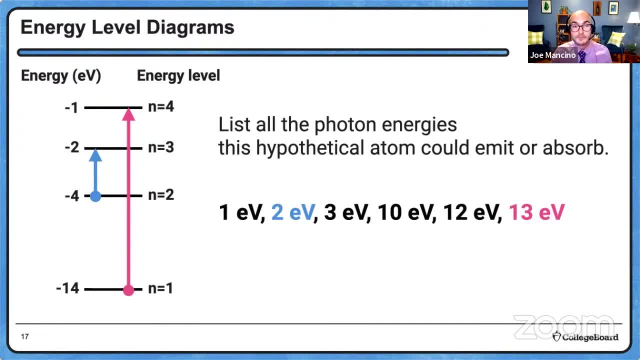 By absorbing 13 electron volts. All right, Let's see if you're still in practice on this. Can you calculate the wavelength of those photons? Well, you're probably thinking not quickly, Mr Mancino. What am I made of math? I mean, you probably have your trusty calculator nearby. I hope you do. What's yours named? 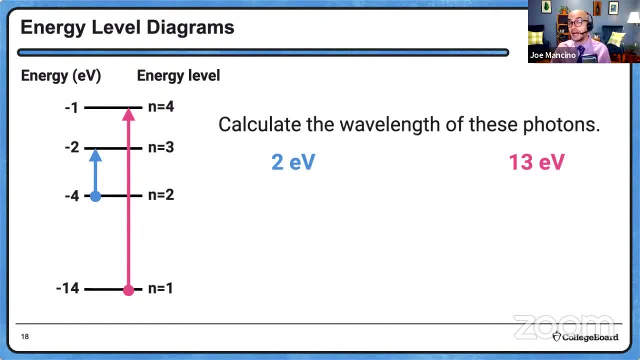 This calculator is really useful. but you know, calculating Planck's constant, multiplying it by the speed of light, that's so annoying. The energy equals HC over lambda, So lambda is HC over the energy. But as you saw in the AP Physics 2 equation sheet, Planck's constant times, the speed of light, is a really convenient number. It's 1,240 electron volt nanometers. 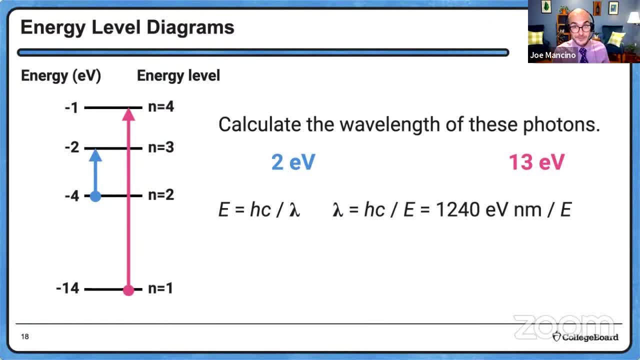 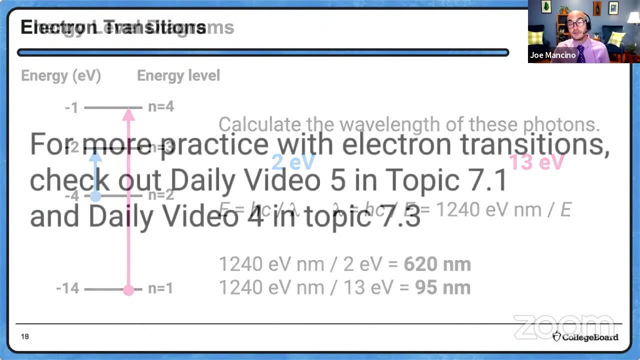 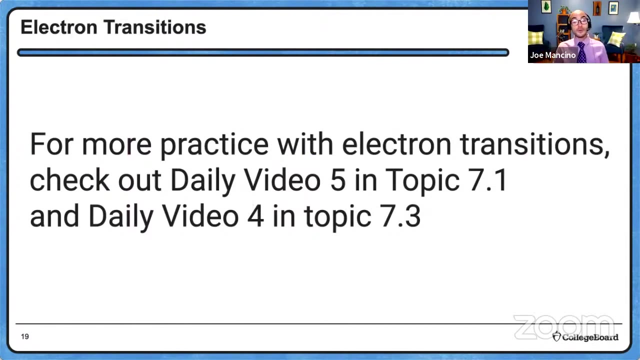 So if we have the energy in electron volts and we use this constant, it'll just give us the wavelength in nanometers, Notice 12.. 1240 divided by 2 is 620 nanometers. 1240 divided by 13 is 95 nanometers. That's really quick, But if you're thinking I need more practice on this, you could check out Daily Video 5 in Topic 7.1 and Daily Video 4 in Topic 7.3.. 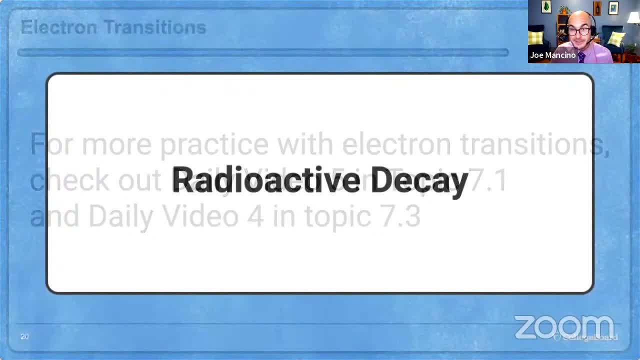 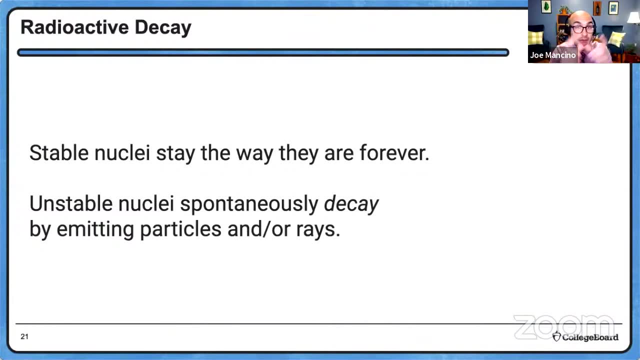 Okay, Next up: Radioactive decay. Well, stable nuclei- good news. they stay that way forever. They're always going to be like that. But unstable, Unstable nuclei spontaneously decay by emitting particles and rays. Some do it quickly, Some do it slowly, Some they might never do it, even though they're unstable, because it might take them more than the lifetime of the universe to do it. 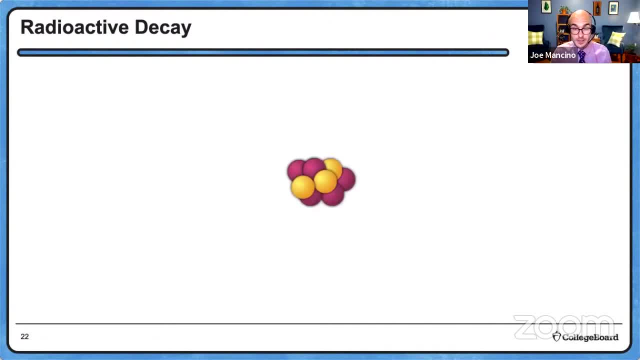 This nucleus, for example, is what we call unstable. Now, when I say unstable, what I'm referring to is that one of those particles in the nucleus is about to change. The nucleus is about to undergo change. It's going to become a different nucleus. Specifically, focus on that proton right there. okay, I'm going to fade the rest of them back in, but that's the one I want you to look at. Watch carefully. It's about to happen. Here it goes, Boom. Look at that. That proton just became something else. And what did it become? That's right. The proton became a neutron. And it became a neutron by emitting one of these called a beta plus particle or a positron. Ooh, fancy. 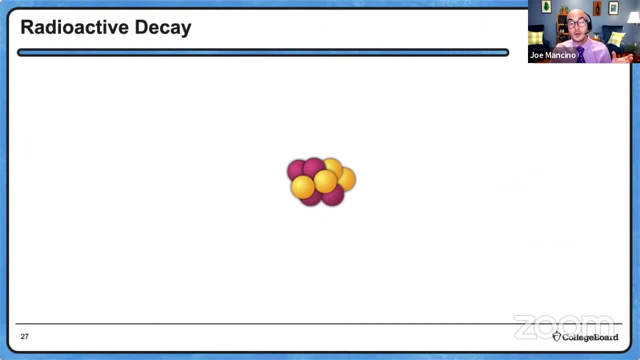 We'll be talking about those in a moment. But this nucleus that's left over with four protons and four neutrons is also unstable. This nucleus, left to its own devices for long enough, will break in half. Now I happen to pick a nucleus that's going to do that really well, basically because I like the way that those two things are called alpha particles. 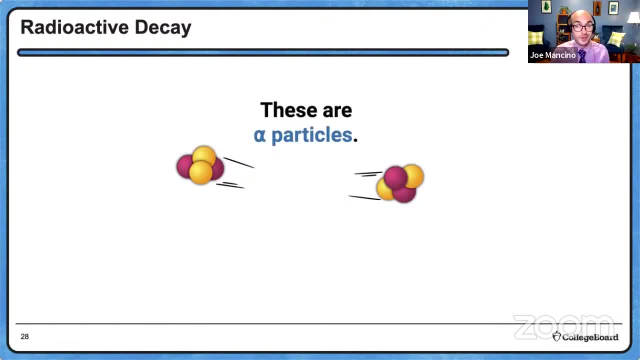 Now, anything with two protons and two neutrons is called an alpha particle. During what's called alpha decay, when a nucleus breaks off into an alpha particle and something else, it also emits a gamma ray. So this gamma ray, this high-energy photon that just jumped off, it's just a really high-energy light ray. 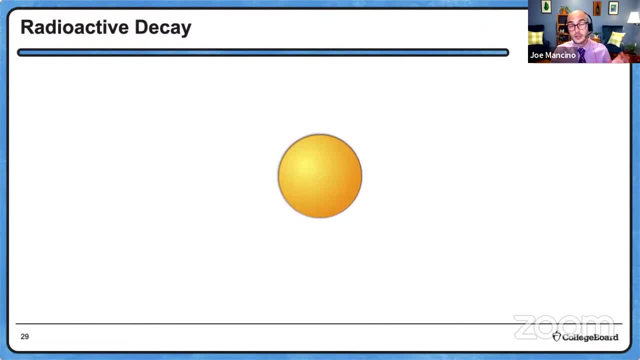 All right, Let's take a look at this neutron. A neutron left on its own for long enough- sorry. a neutron in a nucleus that is unstable can undergo what's called beta minus decay. Now you may have noticed that neutron, it just became a proton. 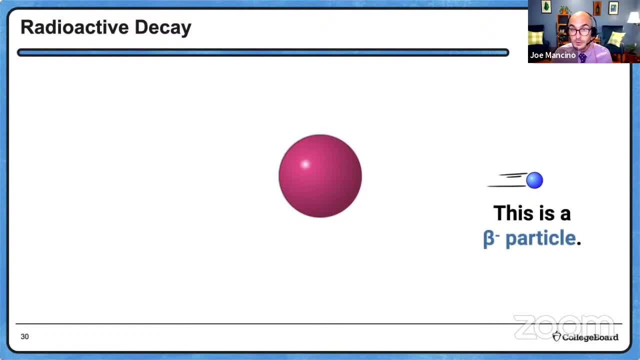 How did it do it? It emitted a beta minus particle. So an unstable nucleus can have beta plus decay, in which a proton becomes a neutron, or beta minus decay, in which a neutron becomes a proton. But now we're going to zoom in even further. 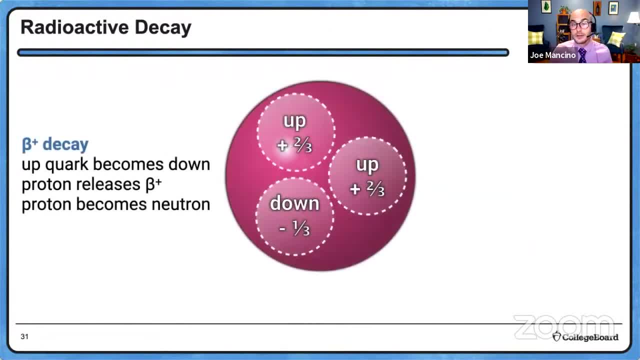 As you learned with Mr Blazo, nucleons are composed of even smaller particles called quarks In beta. In beta plus decay, an up quark becomes a down quark. So focus on the up quark on the right. Watch what happens when it becomes a down quark. 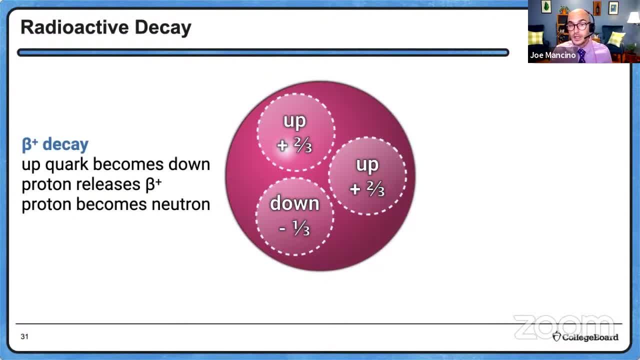 Notice, its charge right now is plus two-thirds. Well, if it becomes a down quark poof, its charge is now minus one-third And that's a difference of one. Let's add those back together, Let's see: Plus two-thirds, minus one-third, minus one-third. 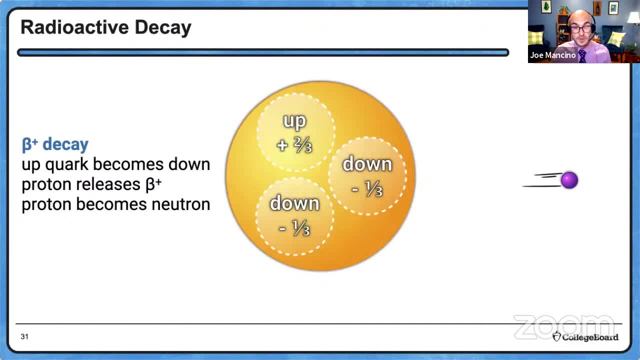 Uh-oh, That is a neutron. So in beta Plus decay an up quark becomes a down quark. A proton releases a positron, a beta plus particle, and the proton becomes a neutron. Neutrons can do that trick in reverse. 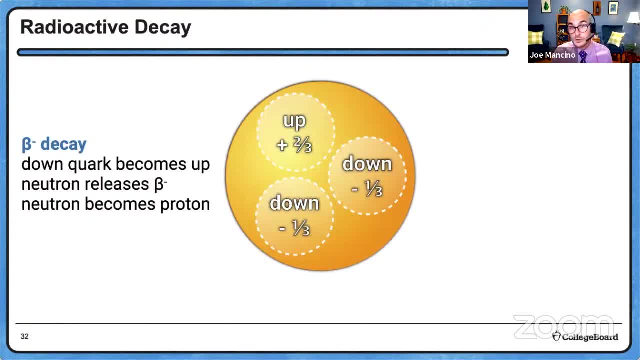 A neutron is composed of two up quarks and a down quark, And a neutron in a nucleus can undergo beta minus decay. And check that out. Oh there it goes. There goes an electron, a beta minus particle, In beta minus decay. a neutron. 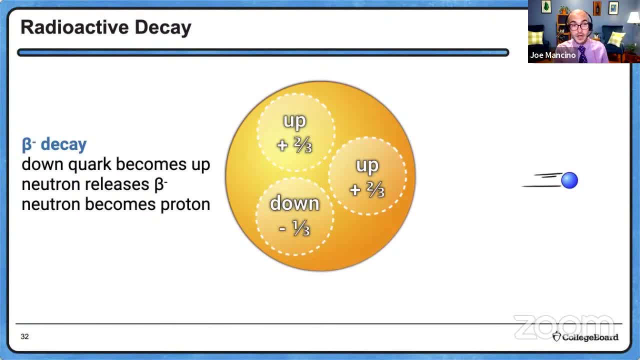 A neutron emits an electron when one of its up quarks turns into a down quark. Sorry, when one of its down quarks turns into an up quark. I said that backwards. A neutron is definitely down, down, up In beta minus decay. one of the downs becomes an up and the neutron becomes a proton. 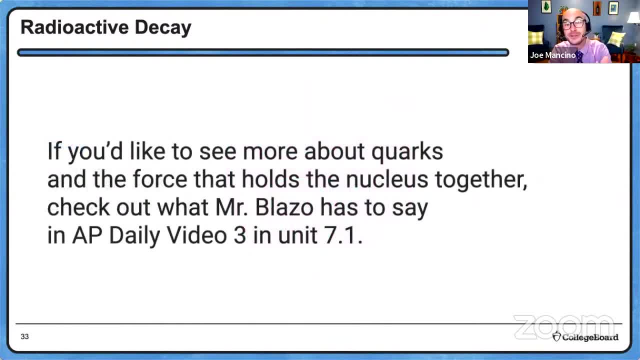 And if you'd like to learn more about that and the force that holds the nucleus together, the strong nuclear force, check out what Mr Blazo says, Video three, unit 7.1.. All right, Quick summary of what you need to know about radioactive decay. 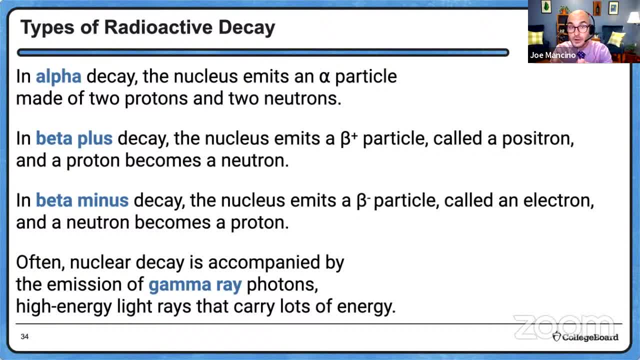 In alpha decay, the nucleus emits an alpha particle made of two protons and two neutrons- An alpha particle, if you like chemistry. you're thinking that's a helium nucleus, And you're right. In beta minus decay, the nucleus emits a beta minus particle called an electron. 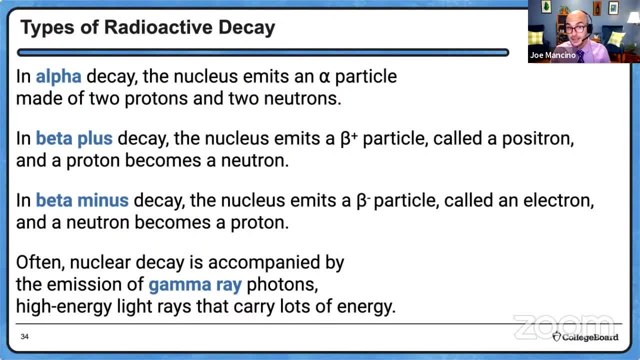 and the neutron becomes a proton. In beta plus decay, the nucleus emits a beta plus particle called a positron, and a proton becomes a neutron, And often nuclear decay is accompanied by the emission of gamma rays, which are just high-energy light rays. 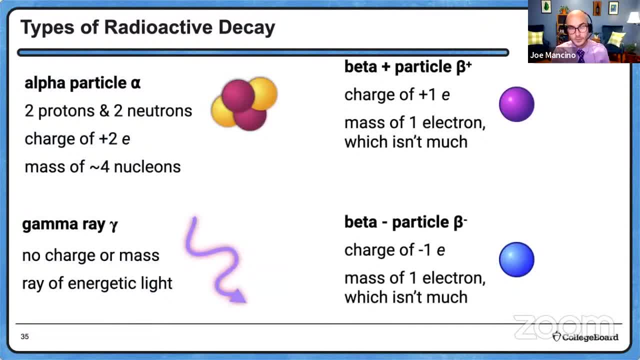 So here's everything that I just said in sort of a bullet point-looking way. You may want to grab a screenshot so you remember these important features of those particles. Let me highlight this. This is what always gets me. As a student, I know I always wanted to talk about the interactions between gamma ray photons and electric fields. 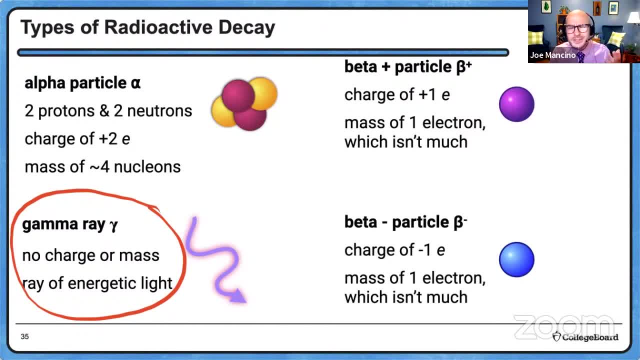 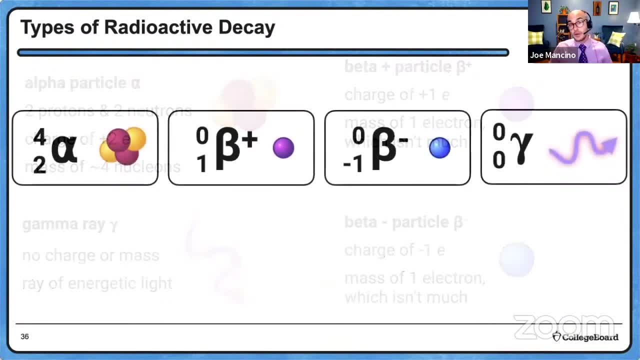 or gamma ray photons and magnetic fields. Well, a photon is just a ray of light. It's not affected by either of those Little Mancino. what were you thinking? Now, if you dig on chemistry, you might prefer to see it written this way: 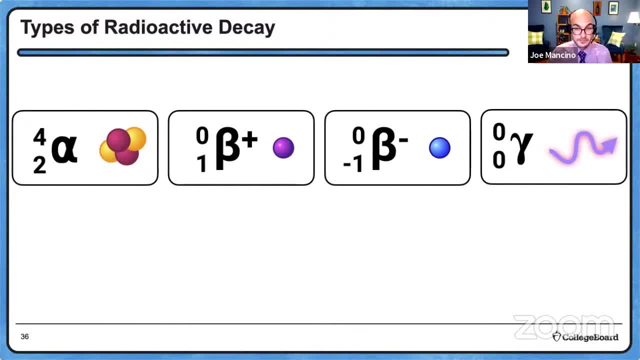 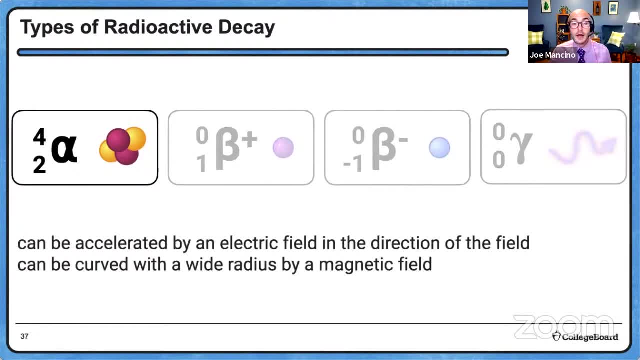 So grab a screenshot of that if it speaks to you. All right, I'm going to fade them out in just a second. There is some information that we need to know about these particles. An alpha particle can be accelerated by an electric field in the direction of the field. 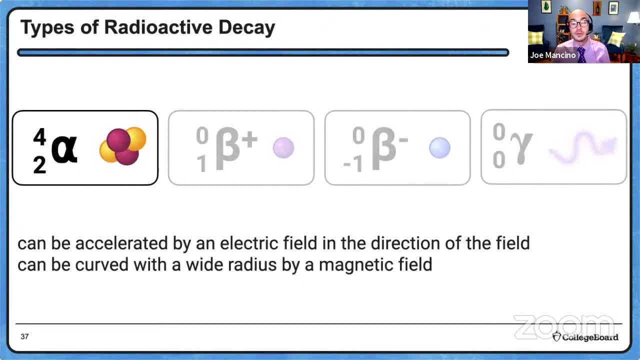 because an alpha particle is positively charged. An alpha particle can be curved with a wide radius by a magnetic field. Lots of mass there. The radius of its curvature will be pretty wide. A beta plus particle, a positron, can be accelerated by an electric field in the direction of the field. 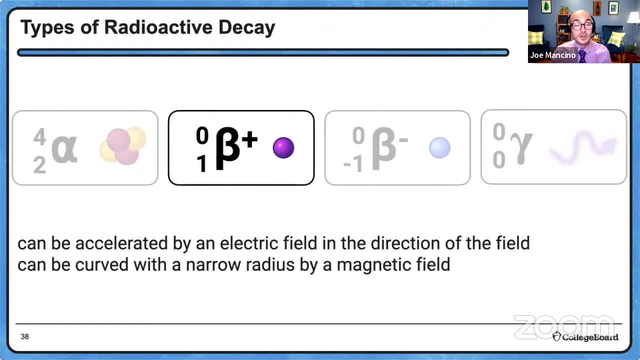 Because it's also positively charged, It can be curved with a narrow radius because it doesn't have a lot of mass. So a positron traveling through a magnetic field will curve in a pretty tight radius of curvature. Hey, same deal with a beta minus particle. 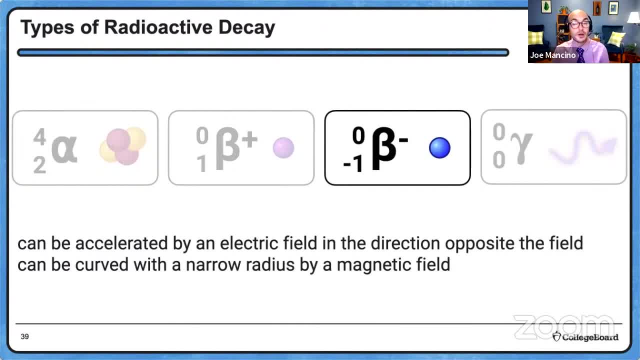 It can be curved by a magnetic field with a small radius of curvature, But it will be accelerated by an electric field opposite the field direction because it's a negatively charged particle. And finally, gamma rays can't be accelerated. They can't be accelerated by an electric field or a magnetic field because it's a light ray. 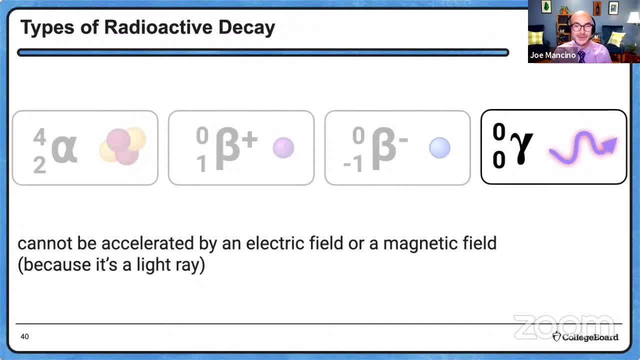 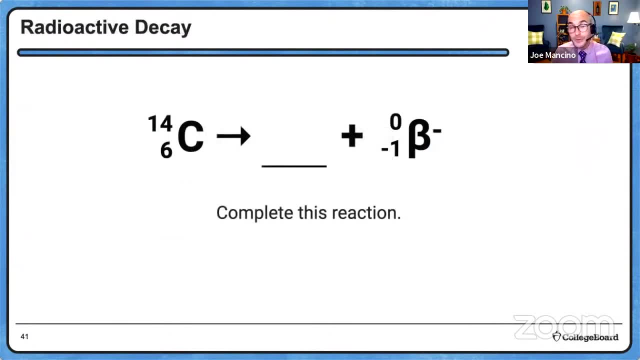 Okay, The other thing that you need to be able to do when it comes to nuclear reactions is a task like this: Complete this reaction Now. we're never going to expect you to have memorized the periodic table and know what the name is of a particular element with a certain number of protons. 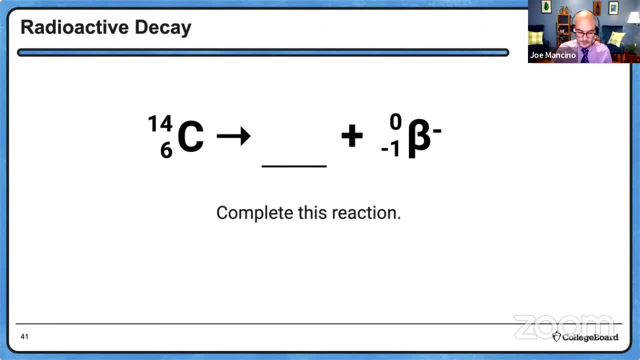 But you should know that well, the total charge and the total number of nucleons is conserved, That if there are 14 nucleons in the beginning, there better be 14 nucleons after the decay. If there's a total charge of six in the beginning, there better be a total charge of six after the decay. 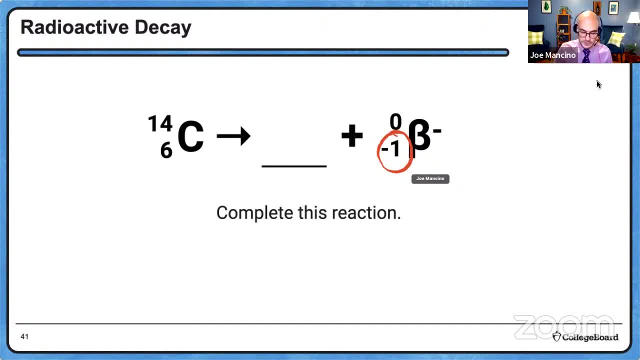 But this beta minus particle has a charge of negative one. So whatever fills this box, it better have a charge of seven, It better have 14 nucleons. Only one thing I know that does that, and that's good old nitrogen. Thank you. 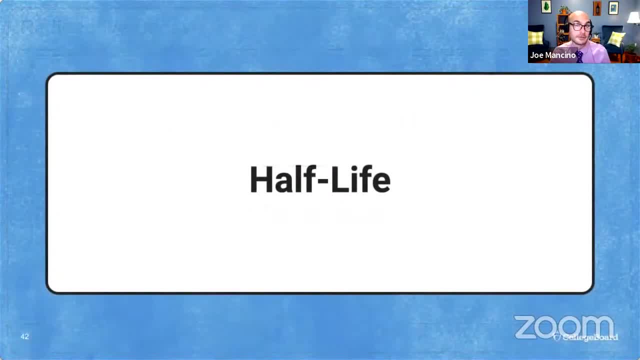 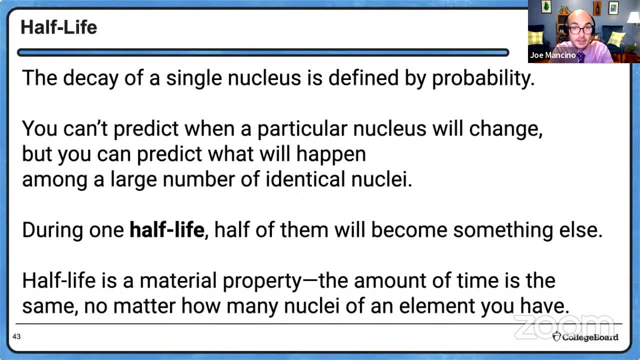 Nitrogen. Okay, folks, it's time to talk. half-life Radioactive decay is a statistical process. The decay of a single nucleus is defined by probability. That means we can't predict when a particular nucleus will change. But we can guess what's going to happen if we have moles and moles and moles of them. 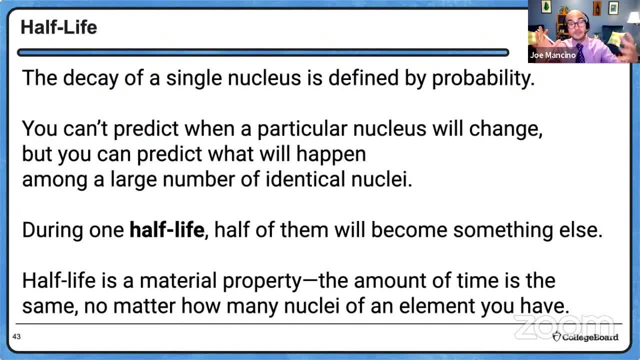 During one half-life, half of our radioactive sample will become something else, will become its byproduct. Half-life is a material property and that means the half-life of a big sample is the same as the half-life of a small sample. As long as we have enough nuclei around, that probability is going to work. half-life of a lot of them is the same as the half-life of a small amount of them. 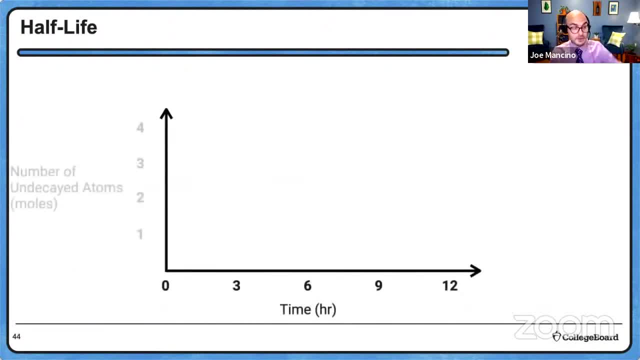 So you, as a smart AP physics student, might have to interpret a graph like this. If you saw my AP Daily video on half-life, you may even recognize some features. You might have to use this graph to estimate the half-life. Well, I see that we start with four moles of undecayed atoms and after just three hours we have two moles. 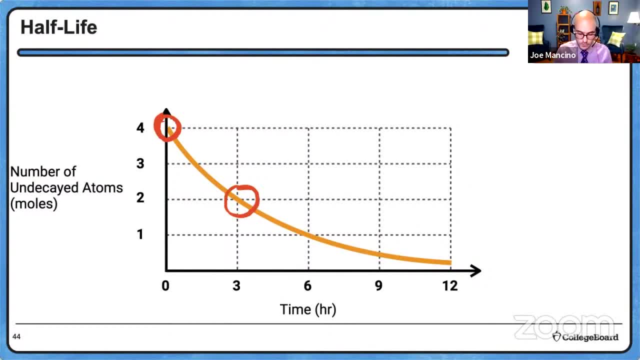 Hmm, All right, we have two moles. After three more hours we have one mole. After three more hours, we have half a mole. After three more hours, we only have a quarter of a mole. That means every three hours there's only half as much left. 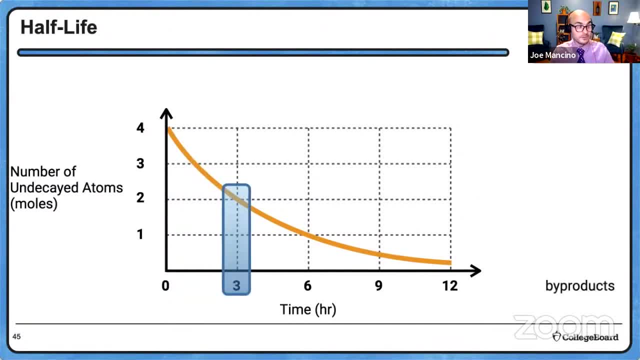 So we start with a full sample After three hours. Well, we have half as many as we started, with half as many undecayed atoms and we have some byproducts. After two half-lives we have even more byproducts, even more and even more. 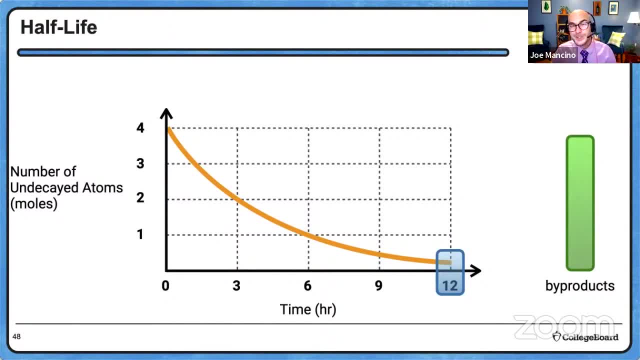 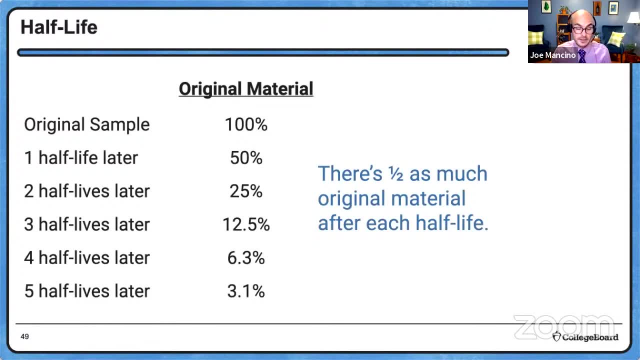 So that I like to think of as kind of the easy mode for interpreting a graph and trying to determine the half-life from the graph. Now you may also see something like this: a data table. Now there may be time in this column. 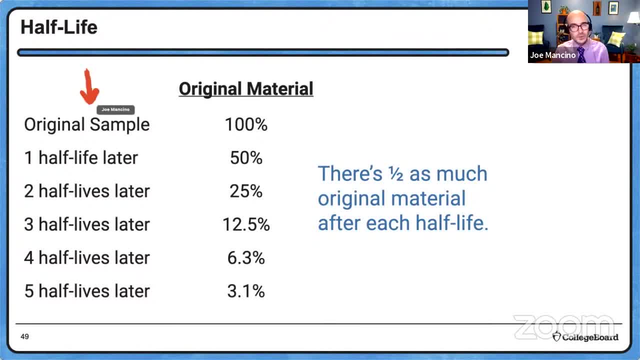 There may be number of half-lives in that column. You'd have to interpret that. But in this case the original material loses half of what was left every half-life. That's the definition of a half-life. But also it tells us how much of that sample is going to be made of byproducts. 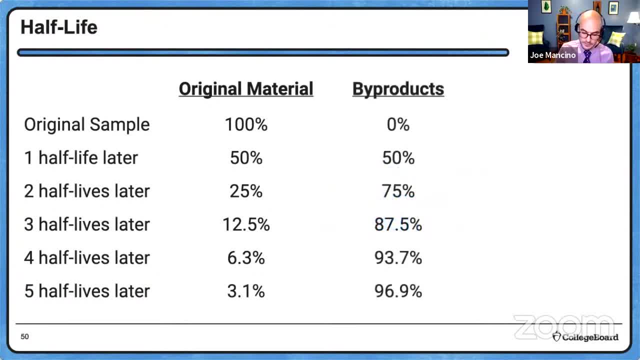 So after no half-lives there's no byproduct, And after one half-life, Half of that sample is byproduct. After two half-lives, 75% of that sample is byproduct. I think it's way more challenging. 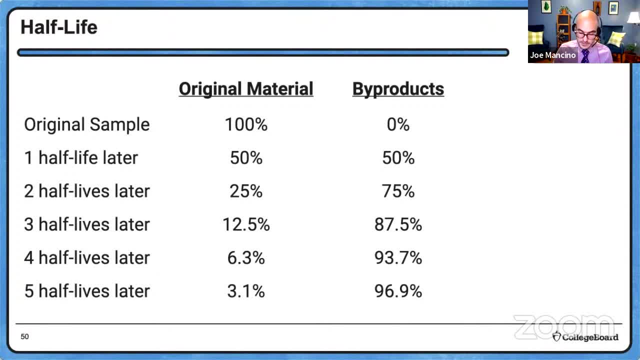 I know it is for me to be given a table like this- pardon me to be given a table like this and asked to predict how much byproduct is left. Or I find it challenging to be given a table like this and predict how much original material is left. 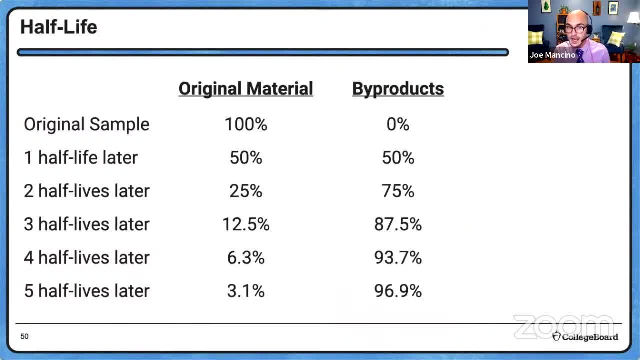 So if you know that that's going to, So if you know that that's going to stump, you, grab a screenshot of this and see if you can answer that on your own. After four half-lives, how much byproduct is there? 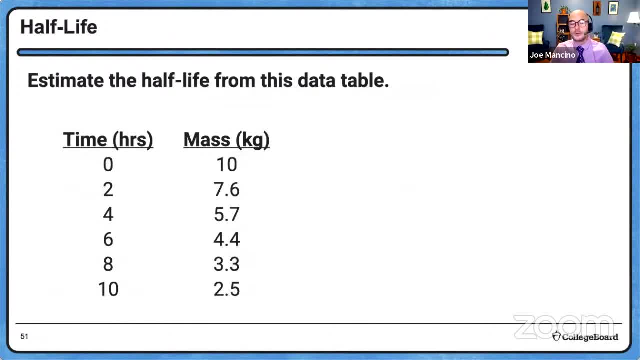 Okay, Can you estimate the half-life from this data table? I'll sip my coffee here. You look at it or hit pause. Remember, half-life is the amount of time it takes for half of the original sample to decay into other half-lives. 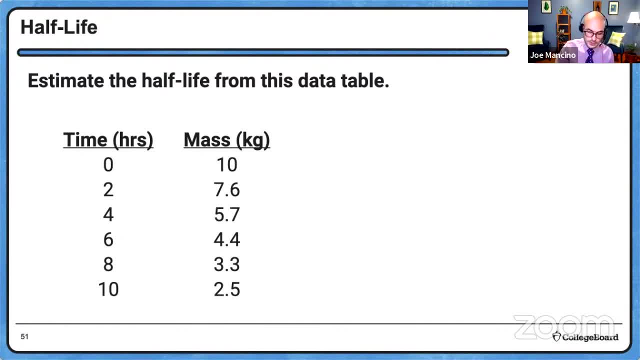 So if you look at this data table, you'll see that half-life is the amount of time it takes for half of the original sample to decay into other half-lives. If we start with 10 kilograms of our original material and then sometime later, there's 7.6 kilograms, 5.7 kilograms, 4.4, well, that's less than half. 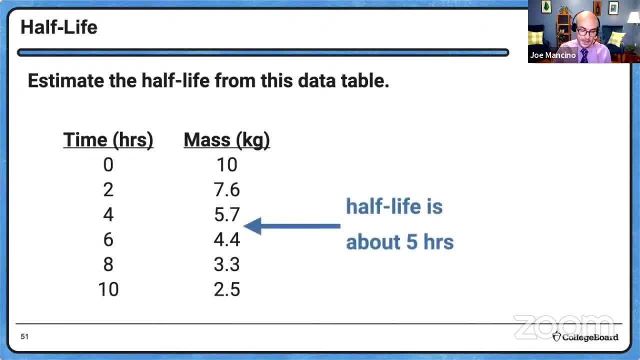 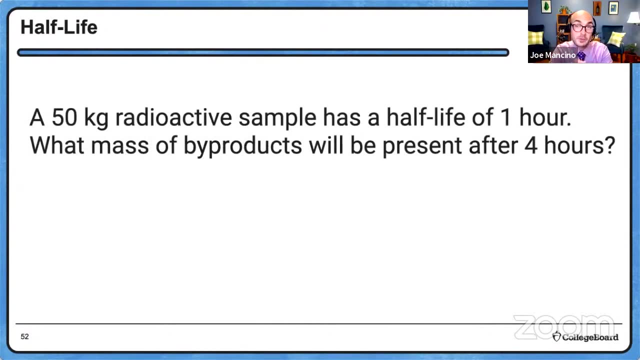 And that means that the half-life is roundabout five hours, somewhere between four and six hours. That's the kind of question that you might see, or the kind of skill that's going to be part of a question. How about this one? a 50-kilogram radioactive sample? 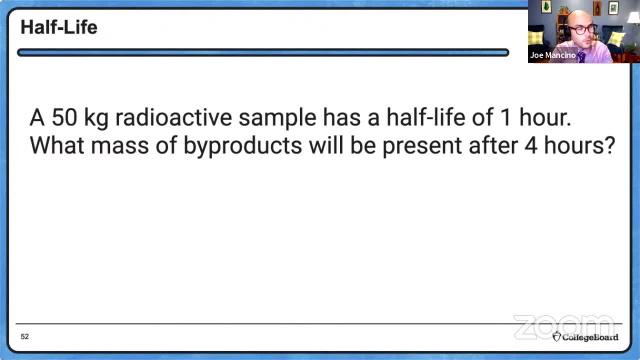 It has a half-life of one hour. What mass of byproduct will be left after four hours? Yeah, that's the tough one, That's the one that I said always gives me trouble, That's rough, And this question is about how much byproduct is left. 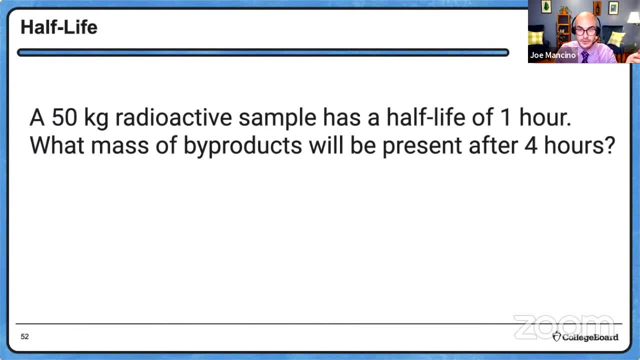 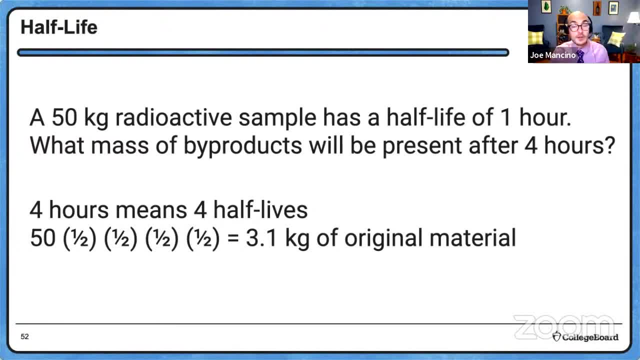 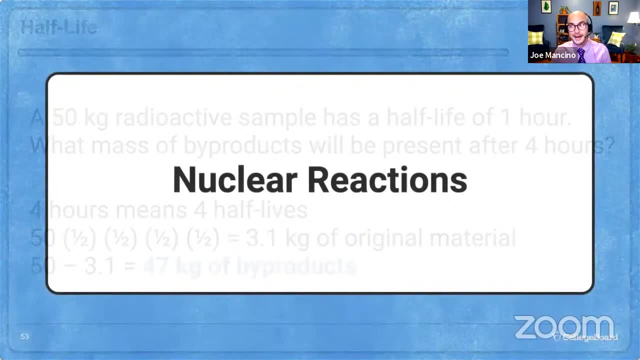 Oh, is that my answer? No, it's not the answer. The answer is that if we started with 50 kilograms and only three kilograms of what's left is our original material, then 47 kilograms represent byproducts. Okay, I know, I talked about the idea of 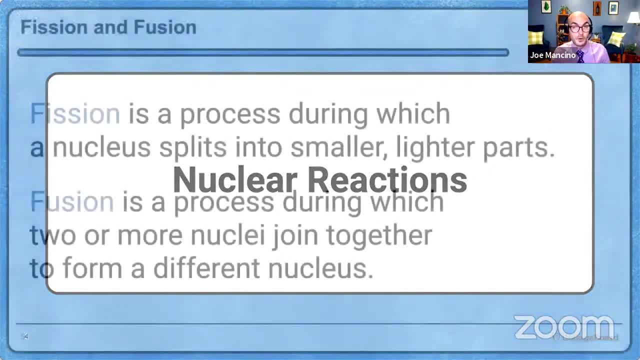 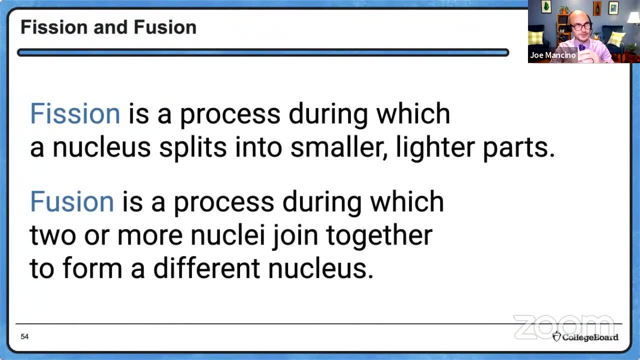 Of balancing charge and nucleon number. but now we're going to delve in a little bit more. as we talk about fission and fusion, Remember, fission is a process of joining, Fission is a process of breaking apart. And fission 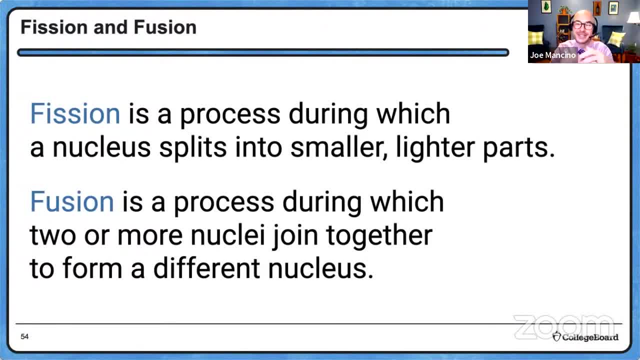 Fission is a process of breaking apart. Fusion is a process of coming together. It's correct on the slide, folks, If you take a screenshot, that'd be great. Fusion is a process during which two or more nuclei fuse join together. 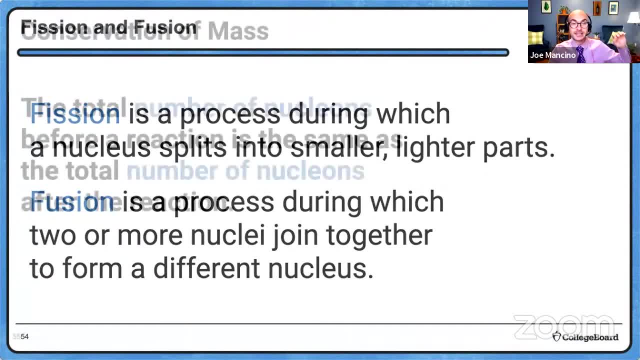 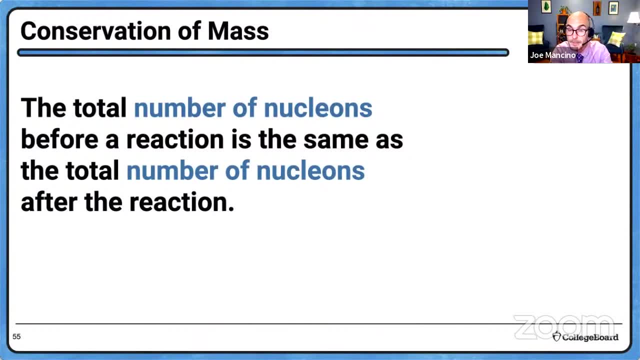 Big idea here. That's why it's going to come up in bold text. The Total number of nucleons before a reaction equals the total number of nucleons after the reaction. Matter is conserved until like 20 minutes from now. 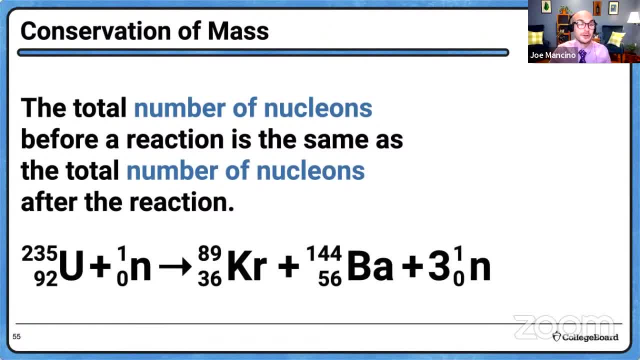 What I mean is: here is a nuclear reaction in which uranium-235 becomes some other stuff. In that reaction- let's take a look at this- The total number of nucleons is conserved. I see 235 here, I see 89 and 144. 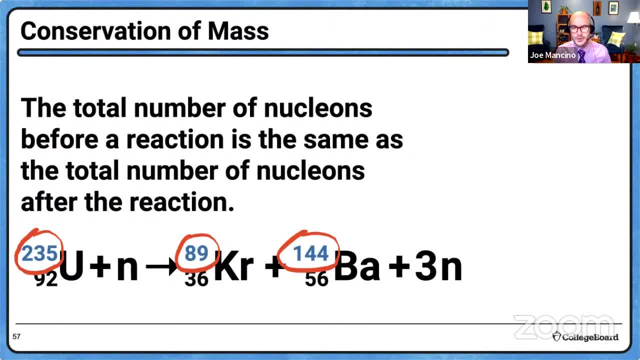 Now wait a minute. 89 plus 144, that's not 235.. Nope, You, as a smart AP physics student, have to remember that neutrons are nucleons. We have to remember there's a secret, invisible one, there. 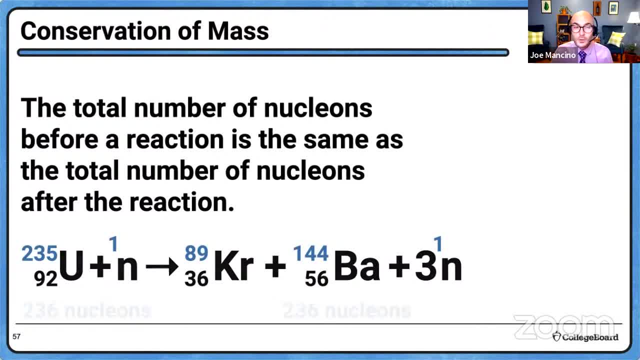 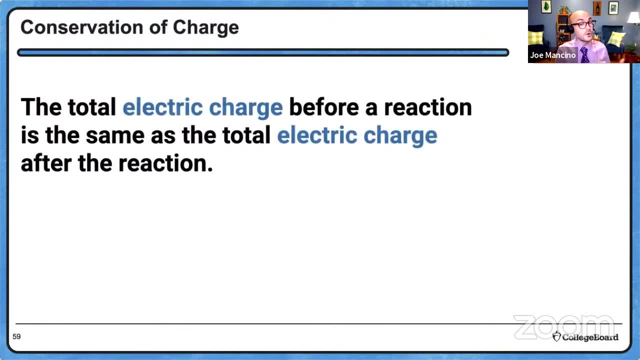 And if we remember that secret, invisible one, we'll see that there's 236.. Nucleons on the left side and 236 nucleons on the right side. The total electric charge before and after a reaction will be the same. Now, that doesn't mean the number of protons will be the same. 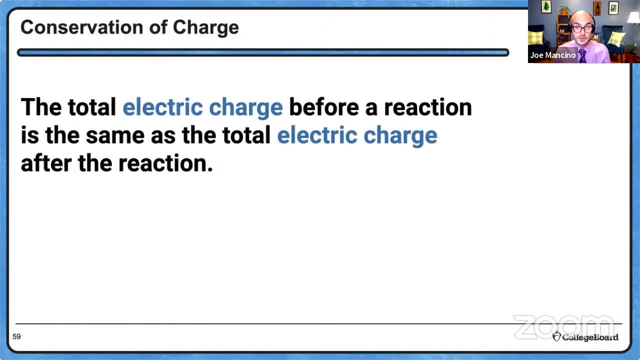 It means the total charge, And Adam's atomic number tells us how many protons there are. but beta-plus and beta-minus particles also do carry charge, For example. let's take a look at this nuclear reaction Notice. before The nuclear reaction, there are 12 positive charges. 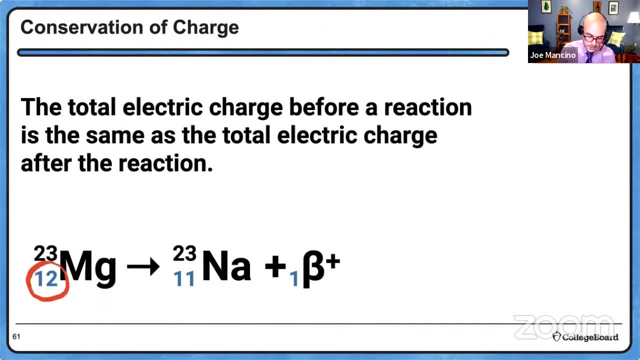 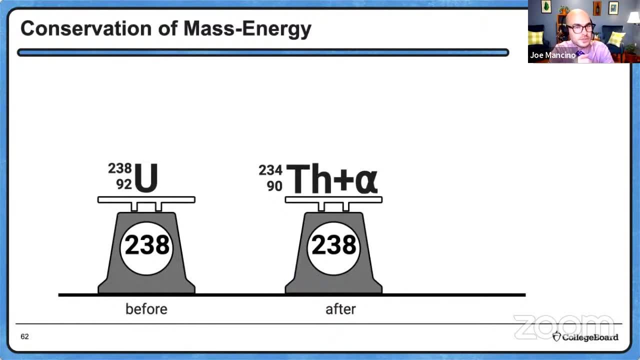 There are 12 protons here, Afterwards there are 11 and a positron. The total charge is conserved. Okie doke, But in a nuclear reaction I said that mass was conserved. It's not quite true. 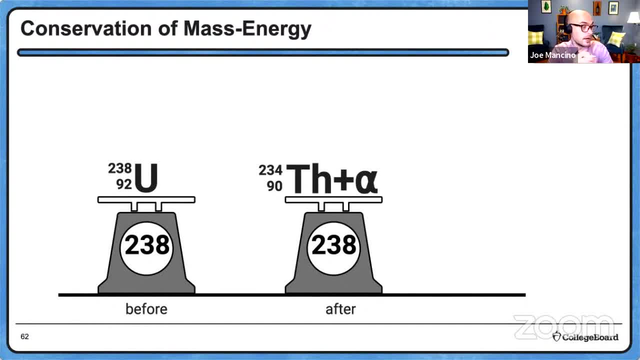 On its surface it looks like mass is conserved. When uranium-238 decays, It looks like the results have the same mass: 238 U's. These are fancy scales that measure single atoms in U's. I should have my department order some of those. 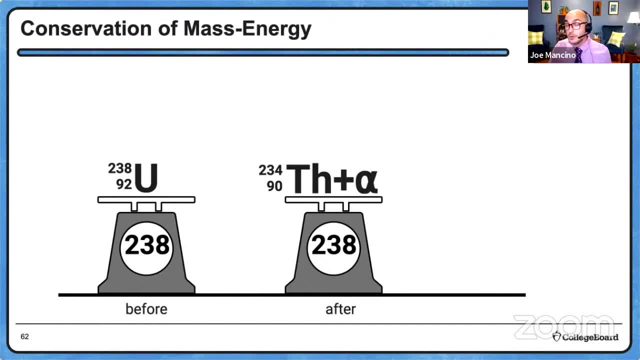 Those things are great And the thing is, as our ability to measure mass historically got better and better, what we figured out is that actually the masses don't add up. Now, a while ago, some of you asked about significant figures and when they matter in AP Physics 2.. 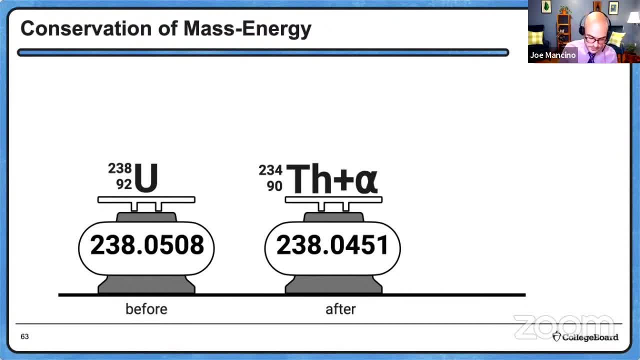 This is when They matter. The first sig fig is the same, The next one is the same, The next one is the same, The next one is the same. And if we were to round this off, that would be the same too. 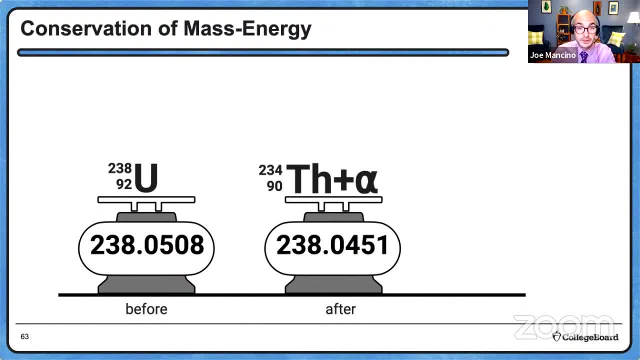 Which means these two numbers are only different in their sixth significant figure. Wow, They're very similar numbers. So when you have numbers for the mass of particles that are making up a nucleus and then the nucleus breaks apart, use all of the detail that you see in that question. 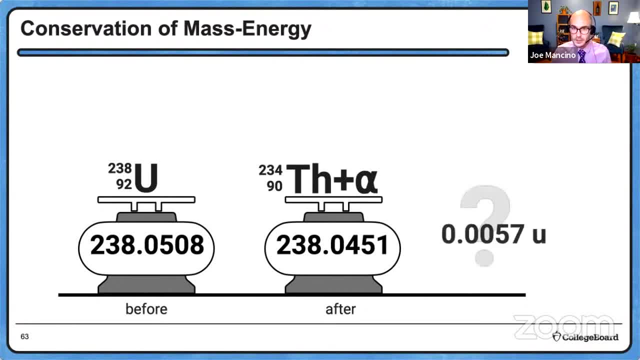 Because, if you do in this one, we notice that, uh-oh, there really is missing mass. Well, where did the mass go? The mass converted to energy And, thanks to Einstein, we can calculate how much energy is released in a nuclear reaction like this. 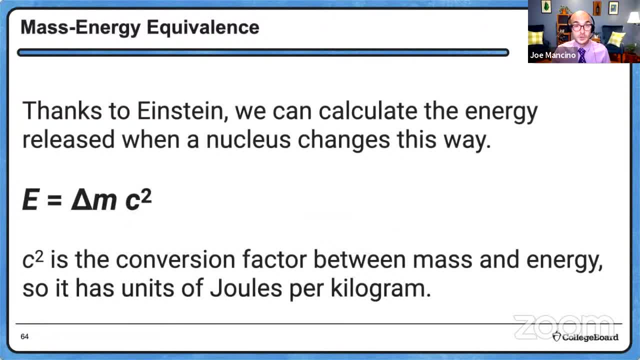 Thanks to Einstein, we can calculate the energy released When a nucleus changes like this. we can use: E equals that change in mass times, C squared. We can use what's called the mass defect, multiply that by the speed of light squared and calculate the energy. 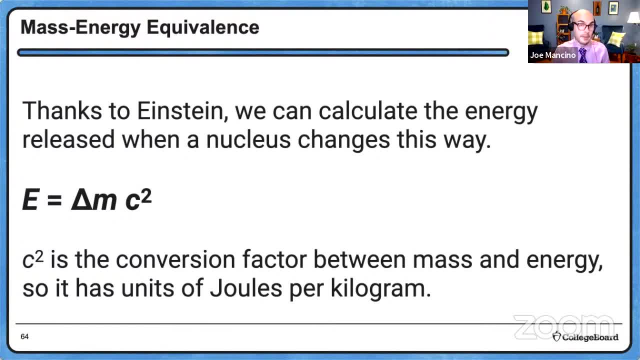 Because C squared is the conversion factor between mass and energy. C squared has units. I know of meters squared per second squared. but that's also equivalent to joules per kilogram. But of course a joule is a really big unit of energy. 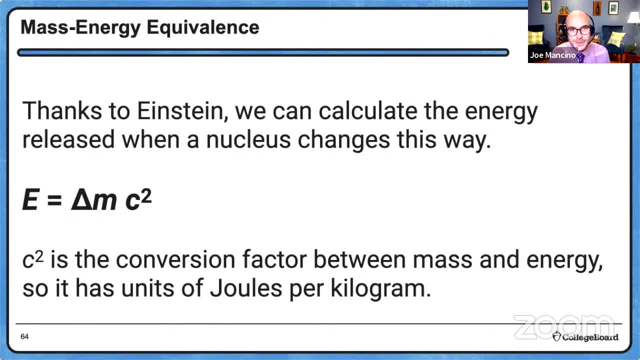 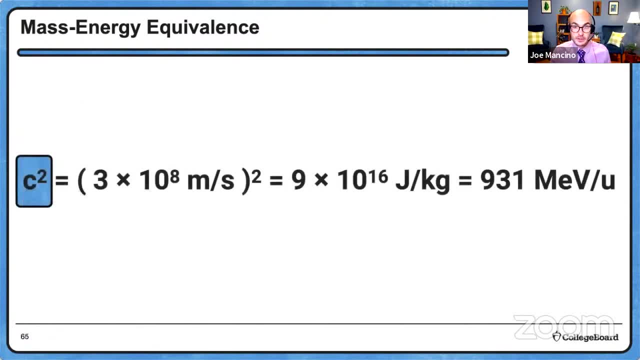 And a kilogram is a really big unit of energy And a joule is a really big unit of mass. We're not going to use those when we talk about atoms. It's way easier to use the small mass unit, uh, MEVs- sorry, the small energy unit of MEVs and the small mass unit of U's. 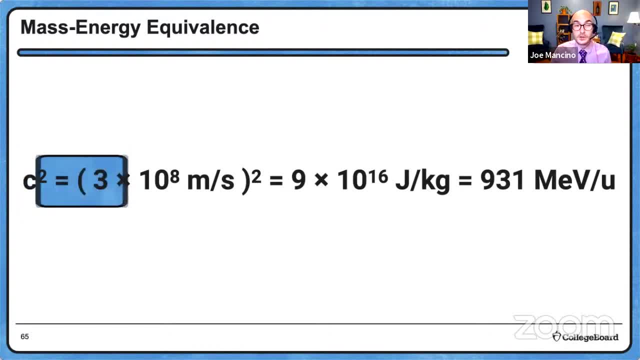 So again 1C squared is also 3 times 10 to the 8th, meters per second squared is also 9 times 10 to the 16th. joules per kilogram is also 910.. So again 1C squared equals 931 MEVs per U. 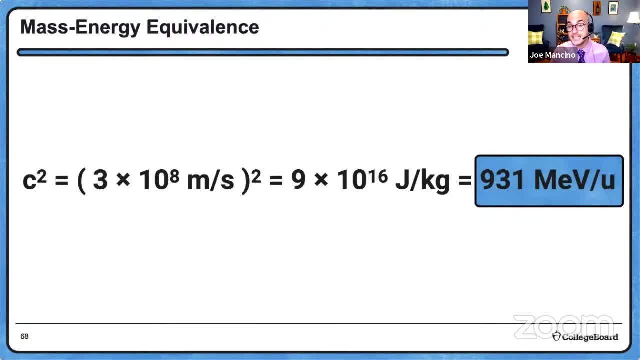 A number so important that it's written right in the table of information. On the AP Physics 2 table of information, you will find C squared equals 931 MEVs per U. That must be important, So let's go back to this. 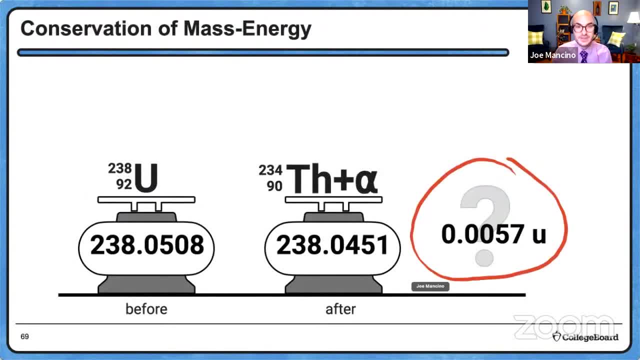 You see this .0057 atomic mass units, which is a very small amount of mass. If you multiply that by 931 MEVs per U, we find that it's 5.3 mega electron volts. Cool Mass converts to energy. 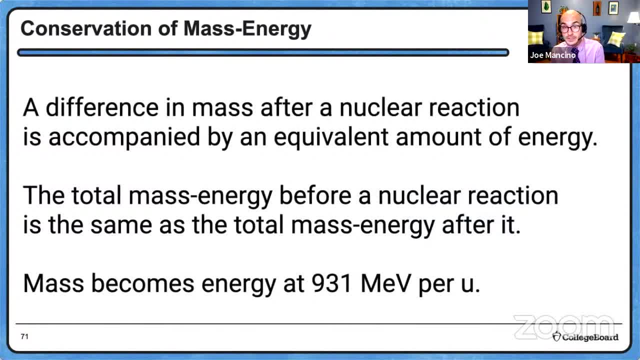 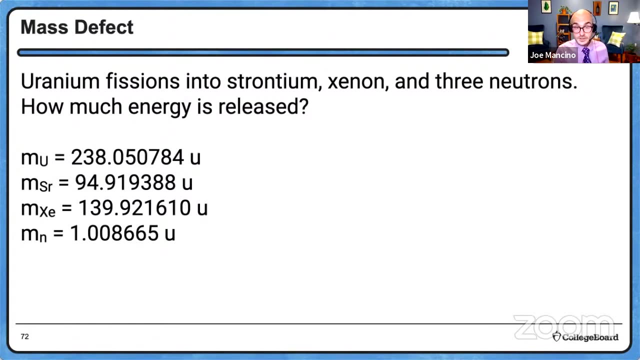 That difference in mass is accompanied by an equivalent amount of energy. but the total mass energy before the reaction is the same as the total mass energy after it. Mass becomes energy at a rate of 931 MEVs per U. Okay, Uranium fissions into strontium, xenon and three neutrons. 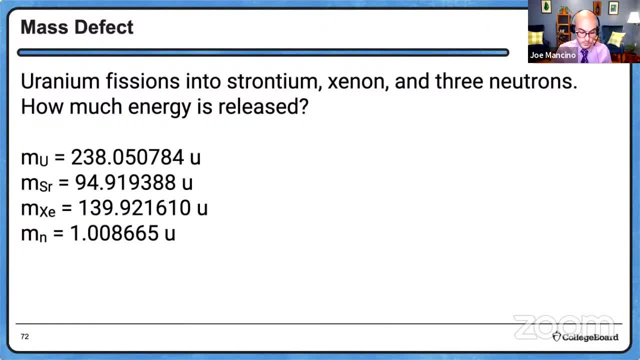 How much energy is released? Oh boy. Well, we have here the mass of one uranium nucleus. We have here the mass of the products, And remember, there are three neutrons. So the strategy for this is to find the original mass, find the final mass, find the difference. 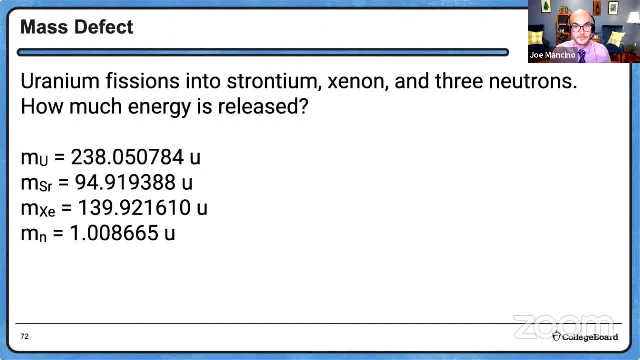 and convert the difference into an amount of energy. Well, I went ahead and did the math, because you know handy-dandy calculator: The original mass is 238.050784.. That's right here. That's just that number there. 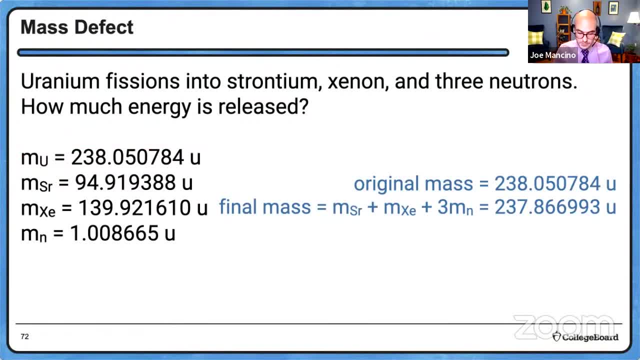 The final mass is the sum of a nucleus of strontium plus a nucleus of xenon, plus three of those neutrons. The final mass is: well, it's less. It's definitely less. So when I subtract those, I see a mass difference of 0.183791 atomic mass units. 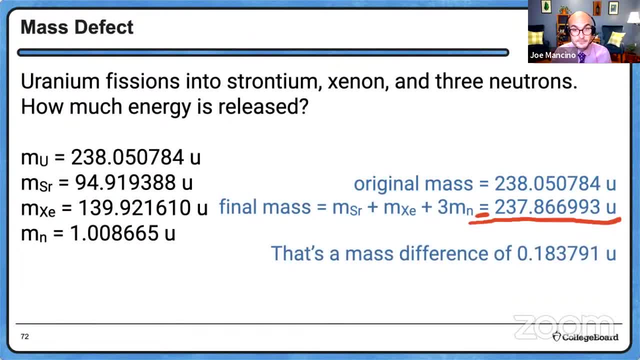 And I know that's a lot of sig figs. This is where they matter. Okay, How much energy is that? Well, if you have your calculator, you can figure it out. Do you remember what to multiply it by to figure out how much energy that is? 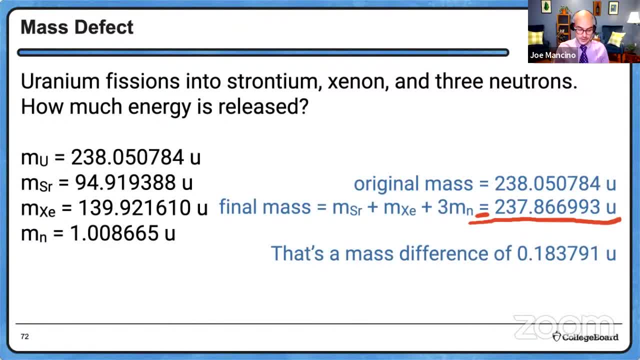 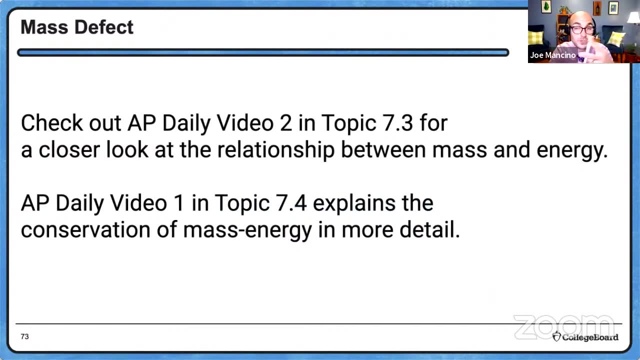 That many U's- I can hear you shouting that from here- Congratulations. It is multiplied by 931, 171 MeVs, But that was a lot and it came really quickly. If you'd like to get more practice with that, check out AP Daily video number two in topic 7.3.. 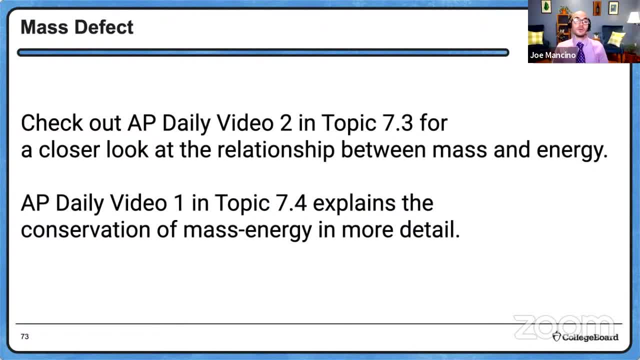 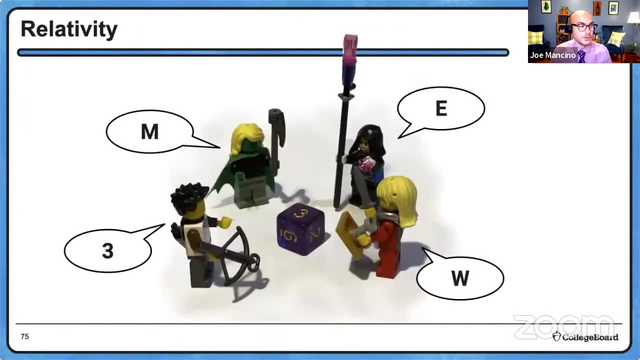 For a closer look at the relationship between mass and energy, Or AP Daily video one in topic 7.4, which explains the conservation of mass energy in way more detail. Finally, it's time to talk about relativity. I could not resist adding this photo again. 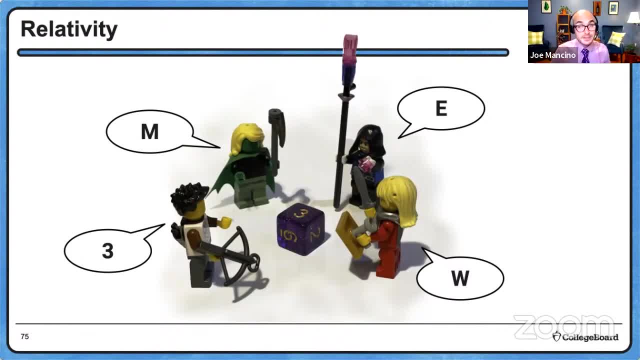 The idea of relativity is that competent observers observing the same event Are not the same event, Are not the same event, can disagree about what they see. None of these observers is wrong. All of them are right in their frame of reference. Relativity has a lot more to do with relative motion, but those are competent. 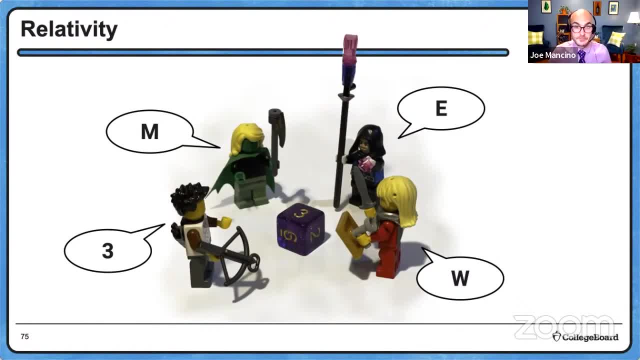 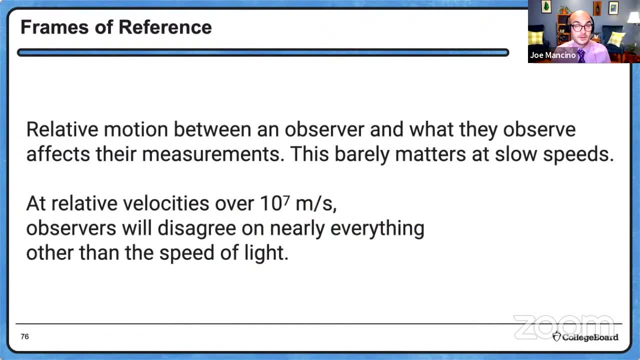 observers. They're all seeing the same thing and seeing it differently. Relative motion between an observer and what they observe affects their measurements, And this barely matters at low speeds, but at what are called relativistic speeds or velocities over 10 to the 7 meters. 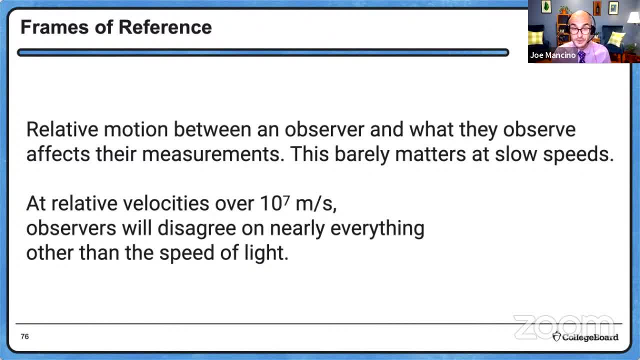 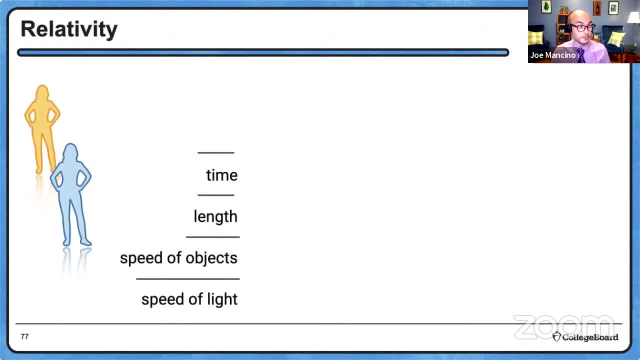 per second. observers disagree on nearly everything other than the speed of light. Well, if you and I were both standing in the same place, I'd say hi. If we had no relative motion between us, we would agree on what time it is and how long things take. We would agree on the. 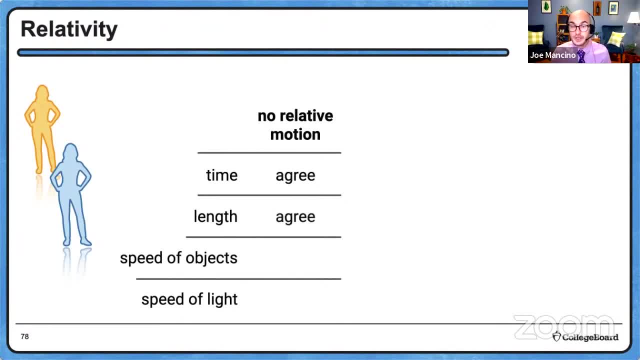 duration of things. We would agree on the duration of things. We would agree on the duration of things. We would agree on the length of objects. If you and I measured something, we're both competent observers- we would agree on the length If you were in my classroom calculating the speed of 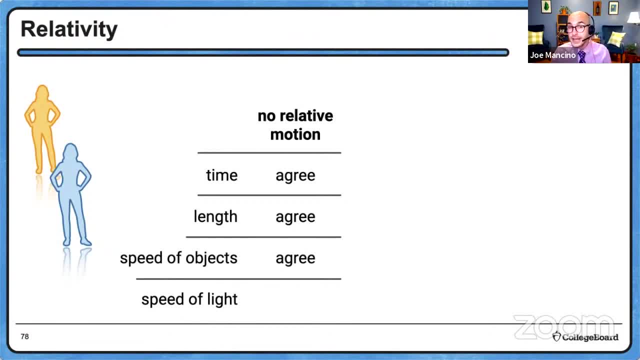 something, we would get the same number. In fact, if we did a lab to find the speed of light, we would get the same number. But if we were moving relative to each other at a speed less than 10 to the 7 meters per second, less than 10 million meters per second, we would still agree on the. 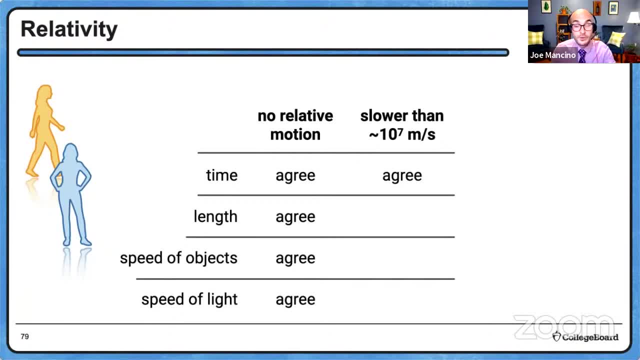 how long things are If we were to measure their length, we would disagree on the speed of objects. We would have some disagreements just because of our relative velocity. We talked about relative velocity in AP Physics 1. Yet we would still agree on the speed of light. I want to draw that. 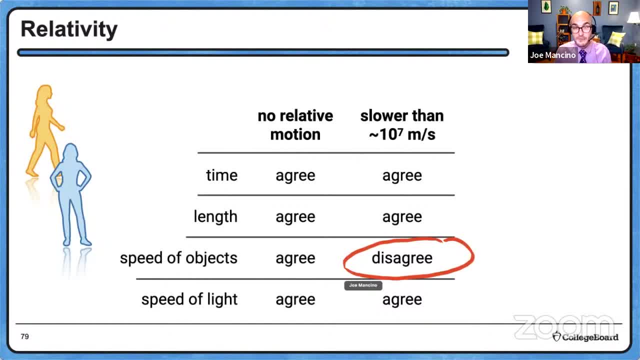 distinction right there, We would disagree about how fast everything else is going to be. We would going, except for light Interesting If we went even faster, if the relative speed between us were even faster than 10 to the 7 meters per second. so if we were approaching what were 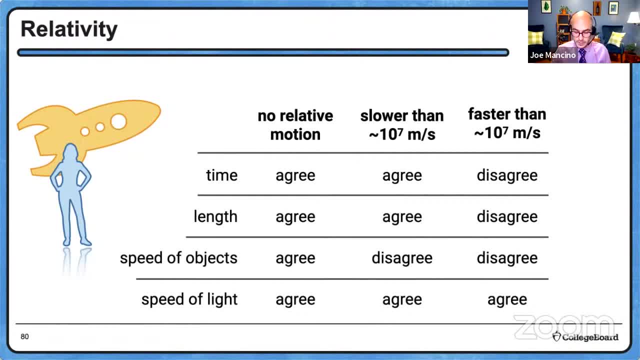 called relativistic speeds. we would disagree about nearly everything. We would disagree about what time it is and what duration of time things take. We would disagree about the length of objects. We would disagree about the speed of objects, But we will always agree about the speed. 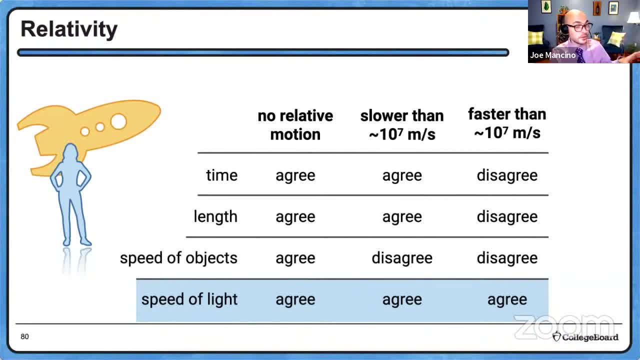 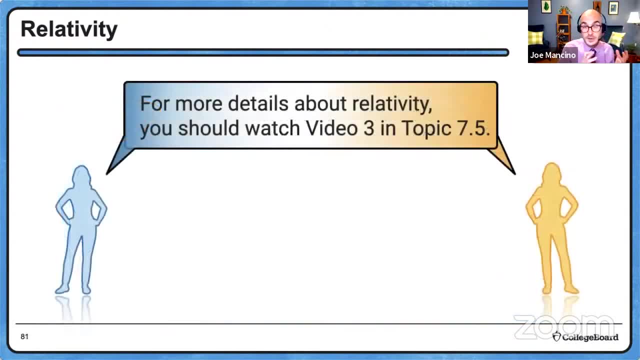 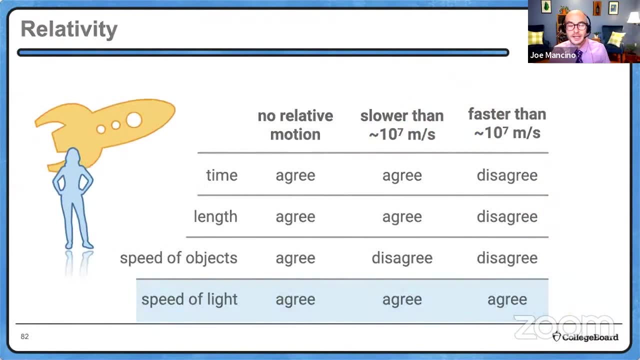 of light. These two competent observers can only agree on two things ever. Thing number one is the speed of light. Thing number two is that for more details about relativity, you should watch video three. But, more importantly, they agree on the speed of light And they also think that they're always. 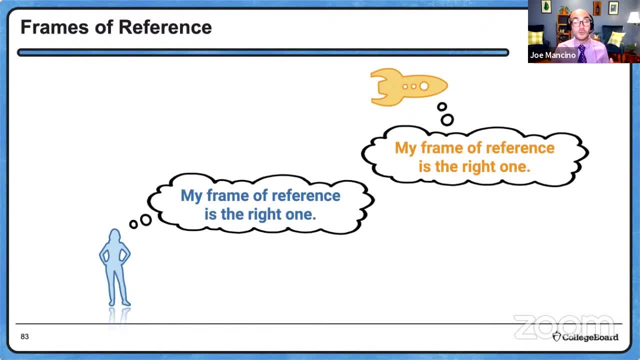 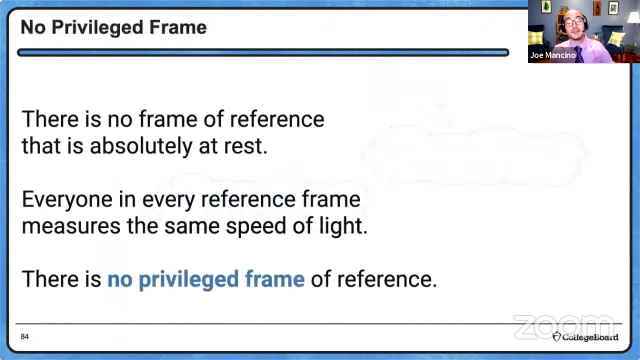 right. They both always think that their frame of reference is the right one. That actually does sound like you and me, But there is no frame of reference that is absolutely at rest. Everyone in every reference frame measures the same speed of light. There's no privileged reference frame. 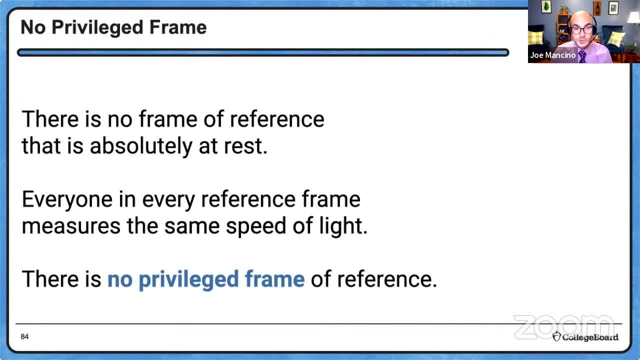 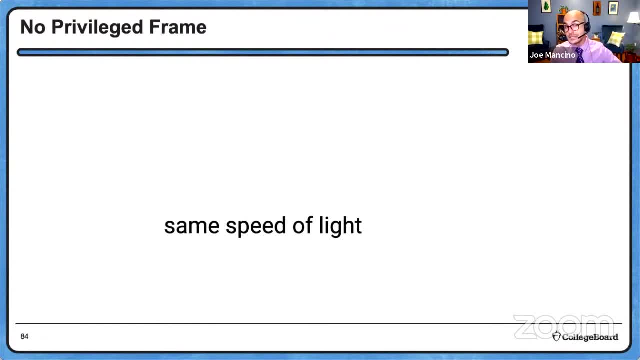 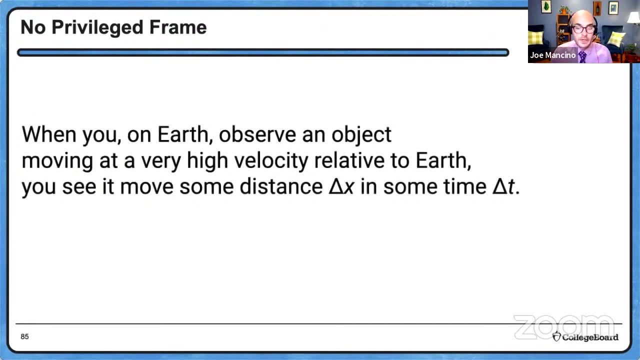 There's no special reference frame, But there is a constant from which we observe motion. We will always measure the speed of light the same way. That is a constant throughout the whole universe. Pretty cool When you on Earth observe- and I don't know why I mentioned on Earth, where else would you be? You're on Earth watching AP. 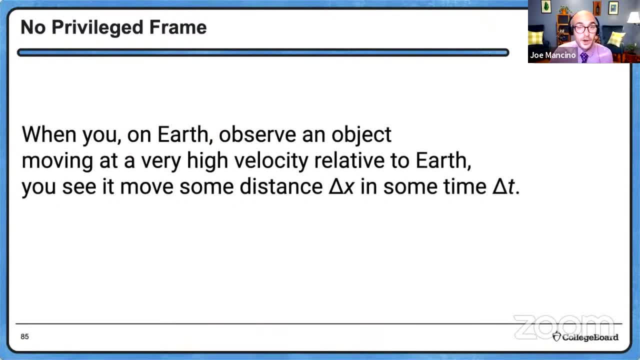 Physics Daily Live review. When you on Earth observe an object moving at a very high velocity relative to Earth, you see it move some distance in some time. You see it move some distance in some time. For an observer, in the object's frame of reference, distance and time are shorter, So the 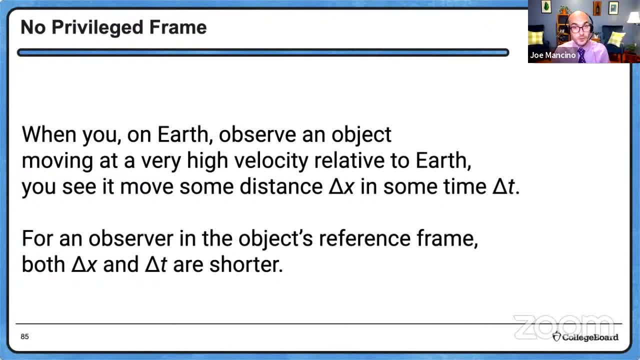 classic example. if you observe someone traveling through space at very high speed and they come back to Earth, they will have aged less than you Because they are moving through time slower than you are. They perceive that less time has gone by. Pretty cool. Now that sounds crazy, but it has been experimentally. 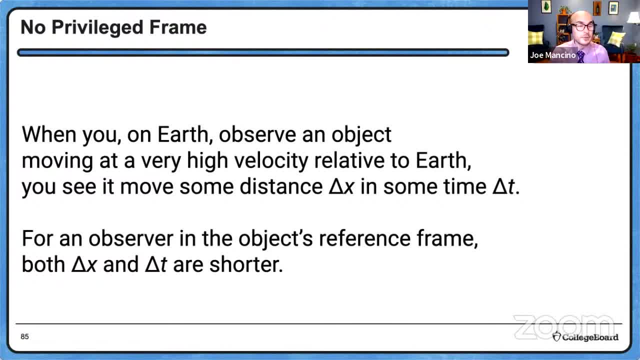 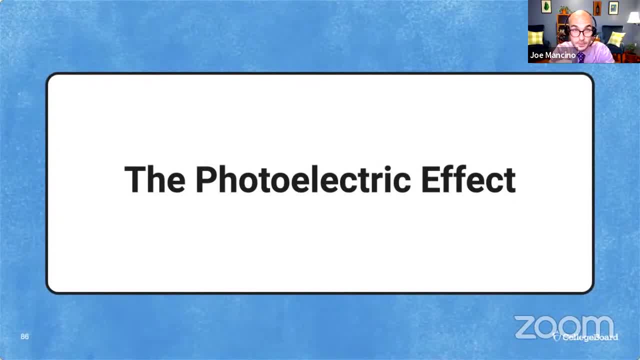 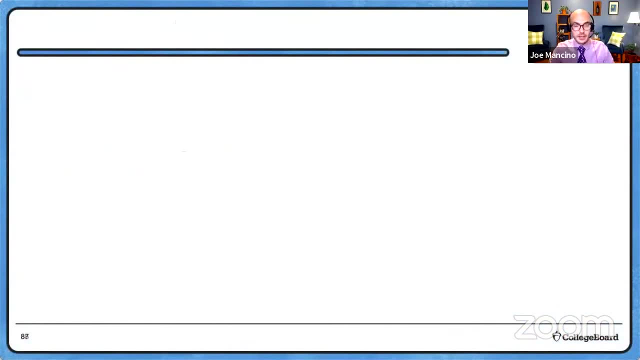 verified. If you watch that AP Daily video you'll even learn a little bit about the experimental verification. But we must move on to the photoelectric effect, the other great example of light's particle nature. The photoelectric effect occurs when light shining on a metal- pardon me- causes electric current to flow through the object. 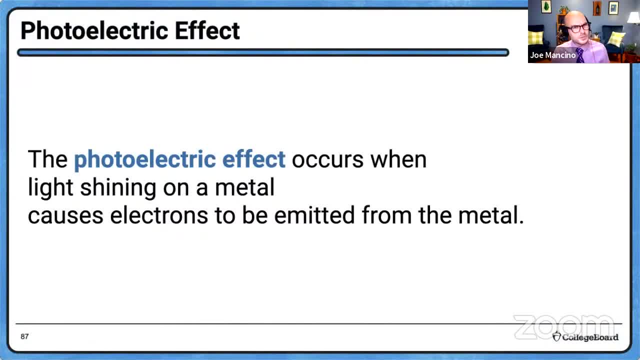 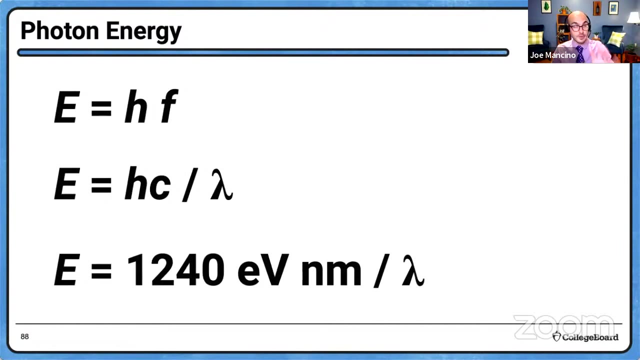 The photoelectric effect causes electrons to be emitted from that metal, which is pretty amazing when you think about it. Light, something that isn't supposed to interact very much with matter, causes metals to emit electrons. That's wild. In order to fully talk about the photoelectric effect, we need to talk about a couple of different ideas. The first one is the energy of a photon. We talked about it a little bit yesterday and a bit more today as we talked about energy levels. 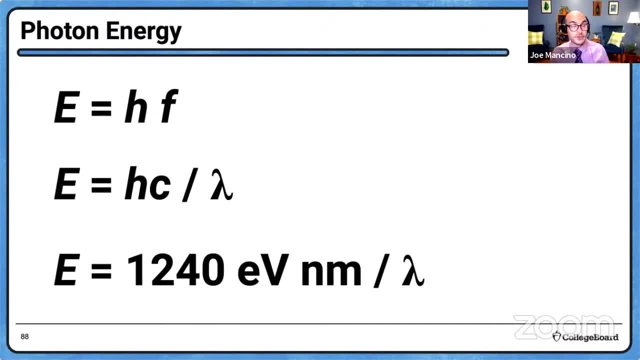 Energy is Planck's constant. So when you're measuring water temperature at a value of 1.1 times frequency, frequency is C over Lambda and HC. is this really convenient constant there? 1240 electron volt nanometers: If you are solving a numerical photoelectric effect problem, you may have really struggled with the idea of calculating the energy of a photon. That's a great way to do it. We also need to talk about the idea of the work function of a metal. The energy needed to remove metal from the möchtee. the energy needed to remove material from the metal is going to be something called a electron effect, which is essentially the function of a metal. So if you're actually using a neutron, you might need to practice that, because we need to try to calculate the energy of a photon. 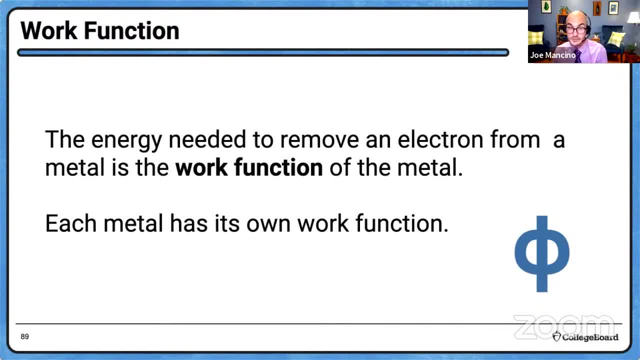 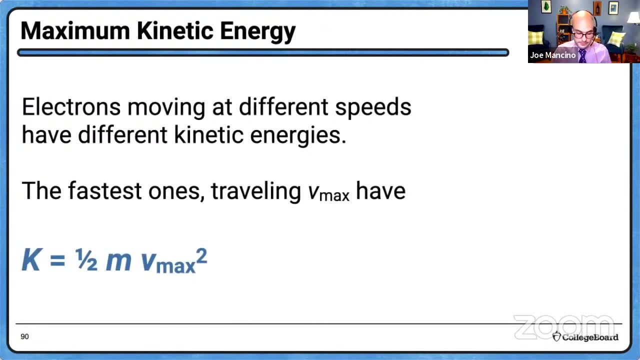 needed to remove an electron from a metal is the work function of that metal. Every metal has its own. That's the Greek letter phi, by the way. Okay, finally, if we have a bunch of electrons, the fastest ones that are moving at v max have the maximum kinetic energy, which is just one half mv. 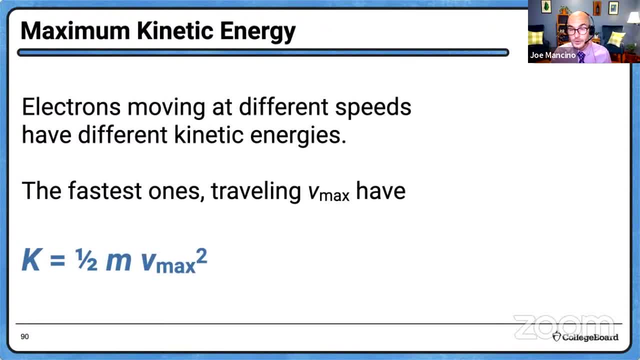 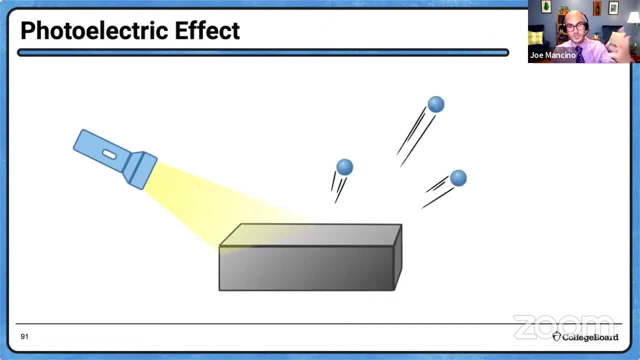 squared All right. the idea of the photoelectric effect is that light click shining on a metal causes electrons to be released from that metal, That light energy. light brings energy to that lump of metal And the work function of the metal determines the energy to get the electrons. 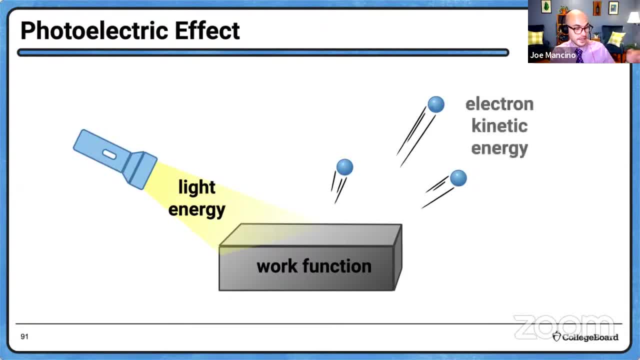 out, And after getting out the electrons have some kinetic energy. So photoelectric effect works Almost the way that you think it would. Energy gets conserved. Light brings energy. minus the work function, the electrons leave with what's left. 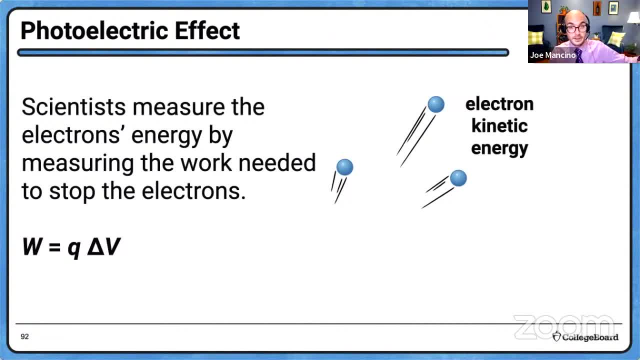 Scientists. by the way, the way that you can measure the kinetic energy of the electrons is by measuring the work needed to stop them. Where work is? q, delta v, as you learned with Mr Strauderman, And that delta v gets a special name when it's used to stop electrons, When it stops. 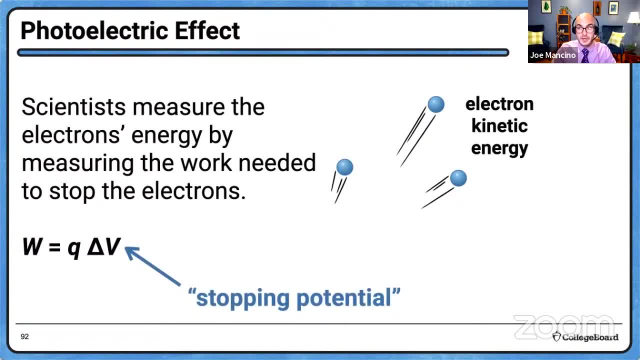 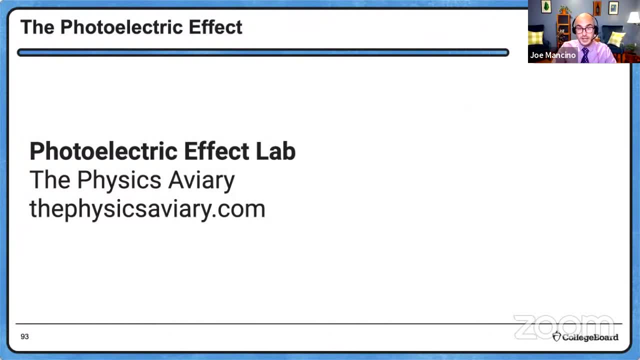 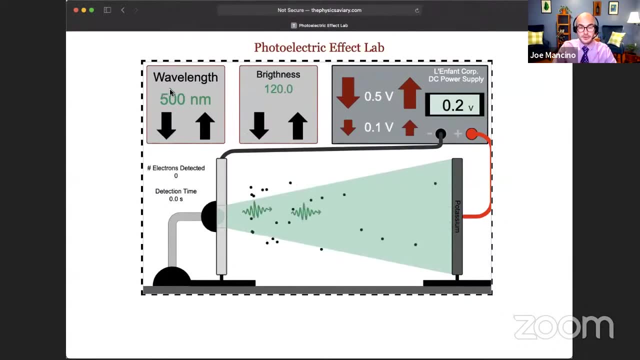 electrons q delta v is called the work function of the metal, And that's the way that you can measure energy. So we've got the movement of the electrons q delta v and q delta v, And I did it, 私 이. �. 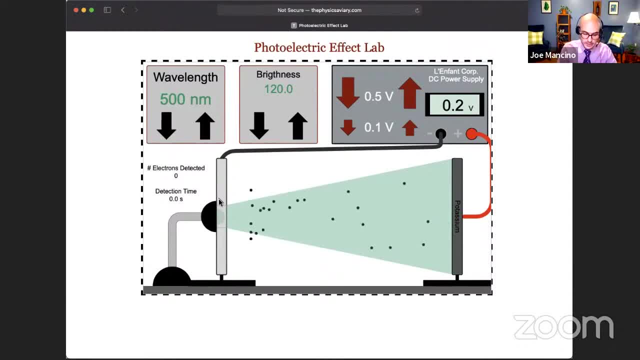 being blasted from this light right here towards that metal surface And those photons are causing electrons to bounce off. Now I have the brightness cranked pretty far. The brightness is cranked up just as high as it can. I'm going to dim this light. 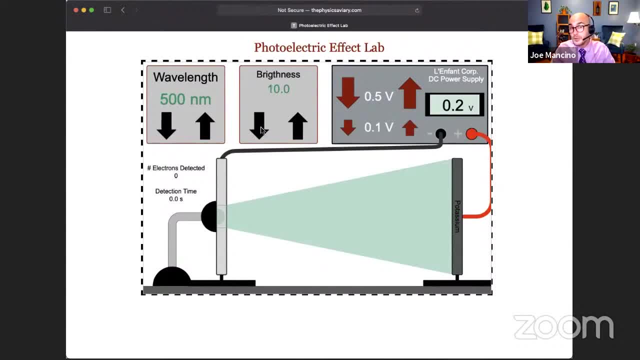 Pretty dim. Dimness means fewer photons per second, And that light is so dim. there are barely any photons, only knocking off just a few electrons. But you'll notice, every photon that strikes the metal releases one electron, And that's important. Einstein's explanation of the photoelectric effect is that one photon knocks off one electron. 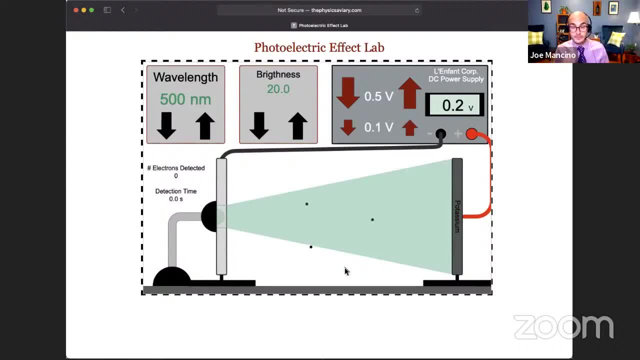 There is a one-for-one correspondence between photons, particles, bundles of light and individual electrons. What you'll also notice is that more photons per second- so this is now a brightness of 120, whatever they are units- way more photons knock off way more electrons. 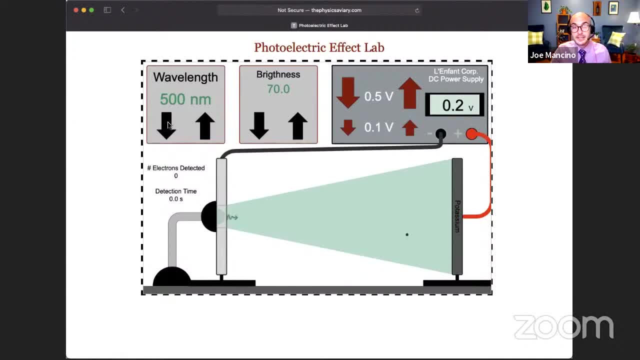 But here's the puzzling thing about the photoelectric effect: Increasing the energy of those photons doesn't knock off a greater number of electrons. Let me make that purple. That's a nice color, Matches my tie. Increasing the energy, so decreasing the wavelength of those photons. 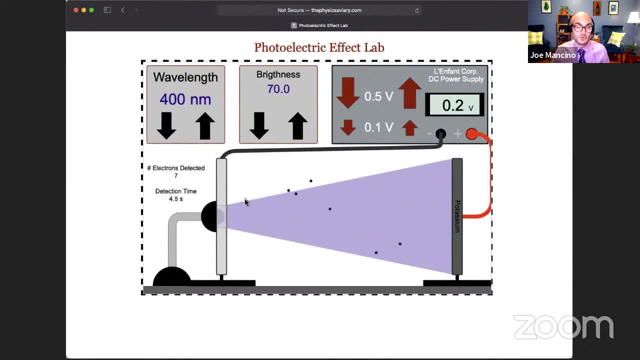 doesn't knock off more. It just makes the electrons move faster. It gives them more energy. I'd have to have a higher stopping potential to stop those electrons. Is that going to stop it? Is 0.8 volts going to stop it? 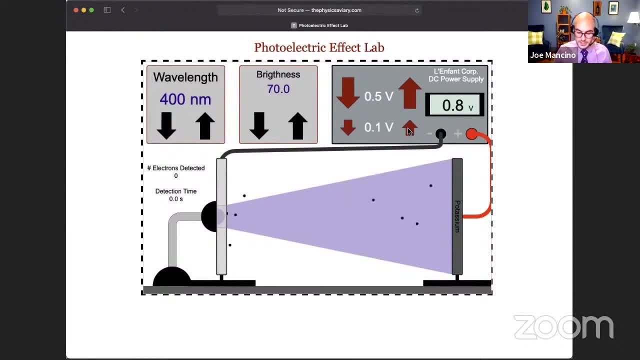 Oh yeah, it is. Look at that. That's the stopping potential. 0.8 volts is the stopping potential for these electrons, Which means, conveniently, the most energetic electrons have 0.8 electron volts of energy. If I were to increase the wavelength, 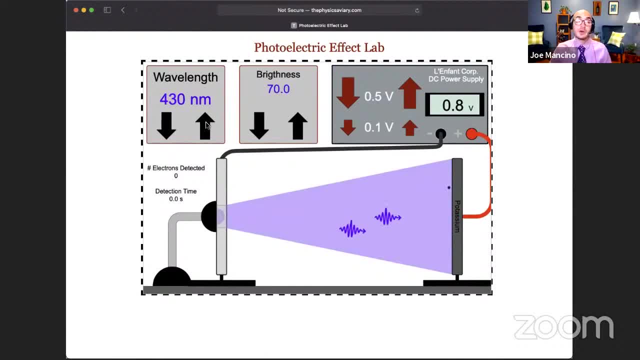 0.8 volts of energy If I were to increase the wavelength. 0.8 volts of energy, If I were to increase the wavelength, none of those electrons would be able to make that jump, Because now the photons have less energy. 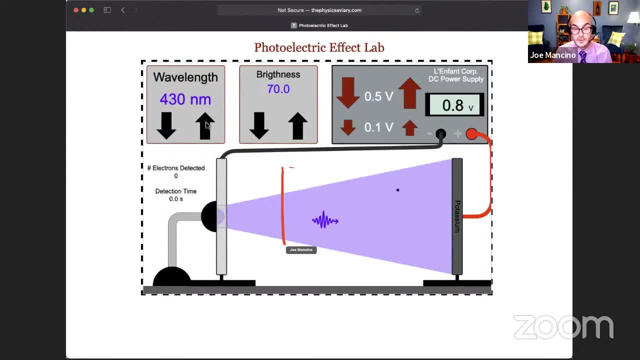 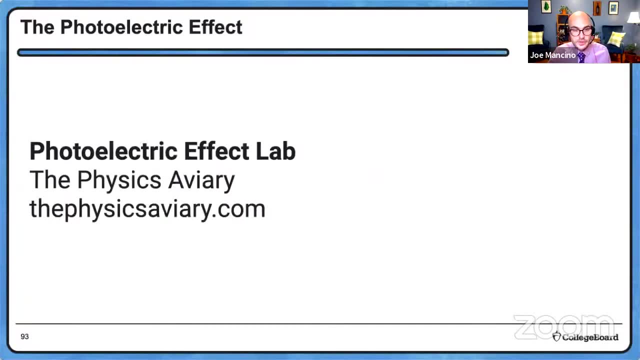 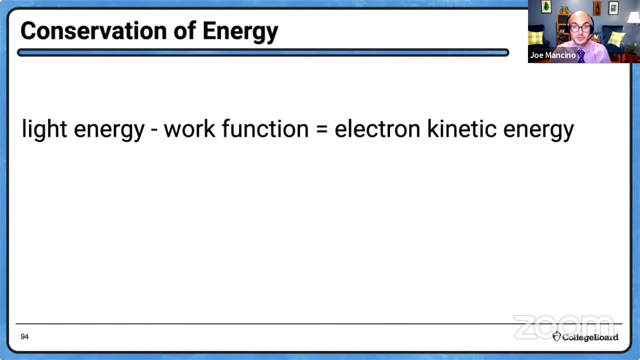 And look, the electrons are all stopping about there. They have less energy. Okay, let's head back to the presentation and wrap things up, folks, Light energy minus the work function equals the kinetic energy of the electrons. There are many ways that we can express that idea. 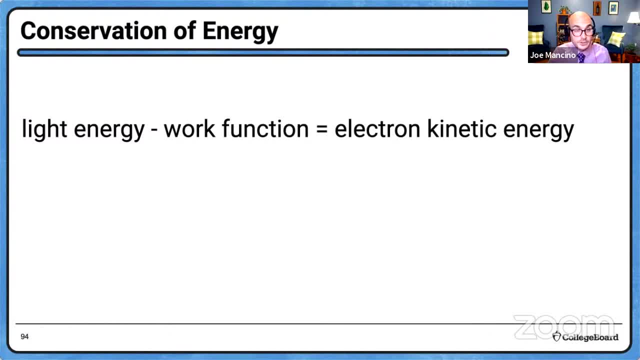 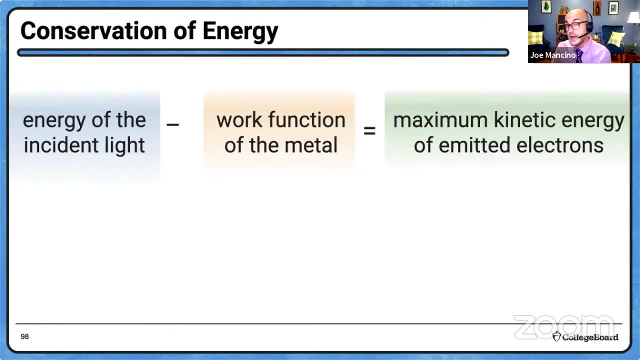 If you watch the AP Daily video about the photoelectric effect, you'll see all the many different ways that we can discuss the energy of the incident light, the work function of the metal and the maximum kinetic energy of the electron. I'm not going to go through the derivation here. 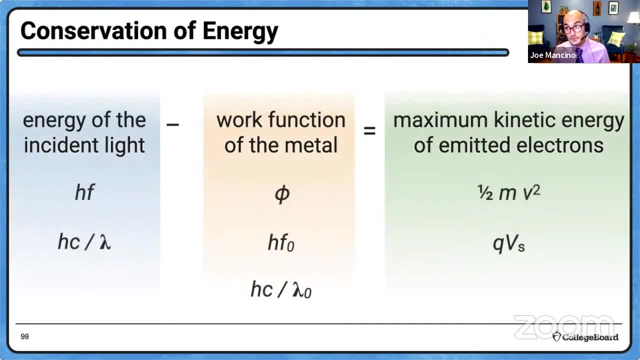 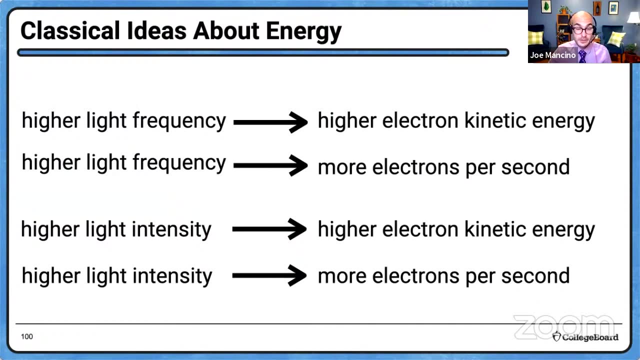 The important part is there are several different ways that we might discuss each of those forms of energy. Also in the AP Daily video about this, I talk about how classical models of the photon and the electron and classical models of the electron and classical models of their energy make predictions that kind of sometimes don't work. 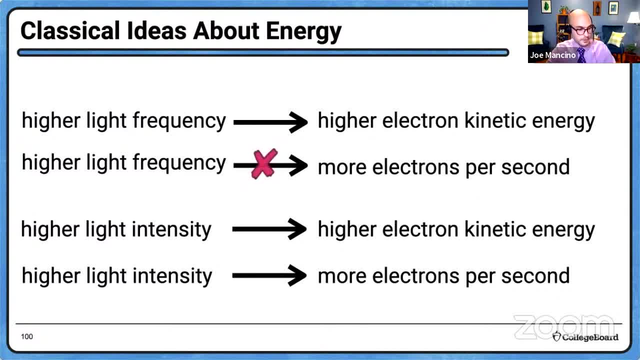 Now certainly, pardon me, higher light frequencies should cause higher electron energies, But classically higher light frequencies could also cause more electrons per second, but they don't. Classically higher light intensity should cause higher electron kinetic energy, but it doesn't. 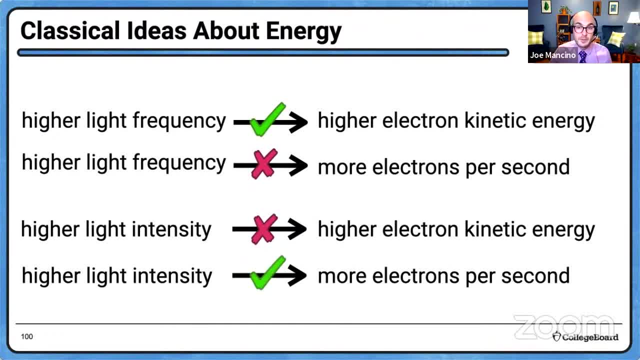 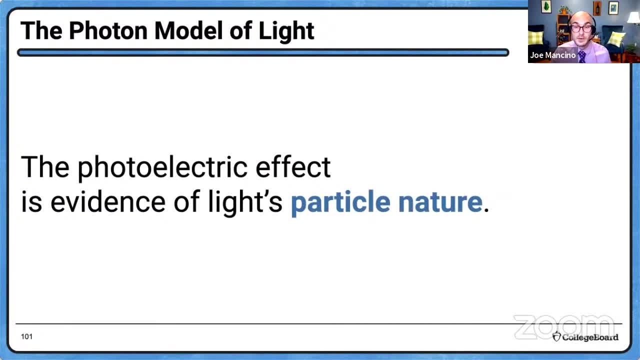 What does that mean? What does happen are those relationships on the top and bottom. So if you'd like to take a closer look at those, you can watch any of the four AP Daily videos in Topic 7.6 that explain how the photoelectric effect is best explained by looking at light's particle nature. 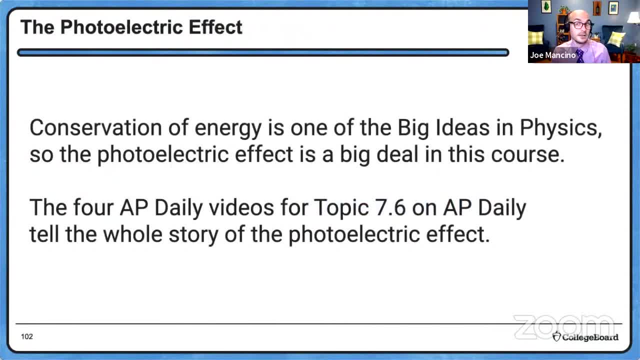 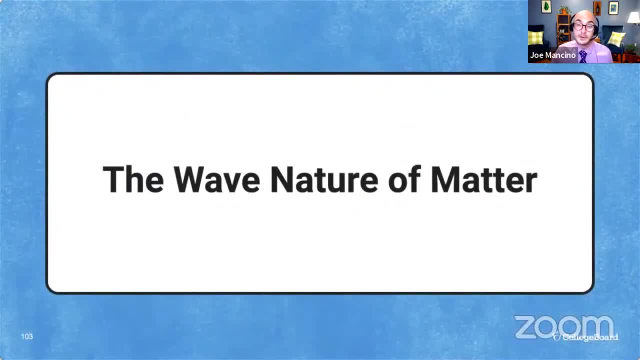 And conservation of energy is one of the big ideas in physics, one of the ones that will definitely be assessed on the exam. All right, we're nearly wrapping it up here, with the wave nature of matter. This is just the idea of diffraction. 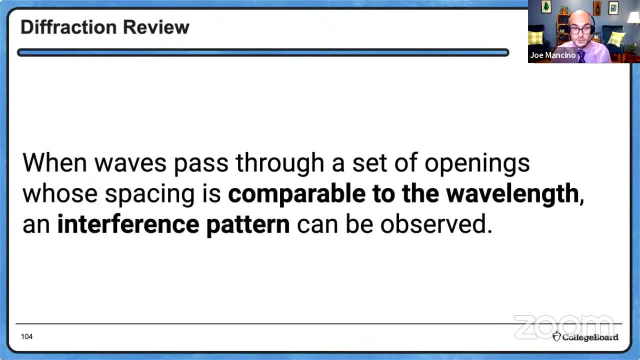 It's what we talked about yesterday. When waves pass through a set of openings whose spacing is comparable to the wavelength, that means between like a tenth of a lambda and ten lambdas, an interference pattern- that's a bunch of maxima and minima- can be observed. 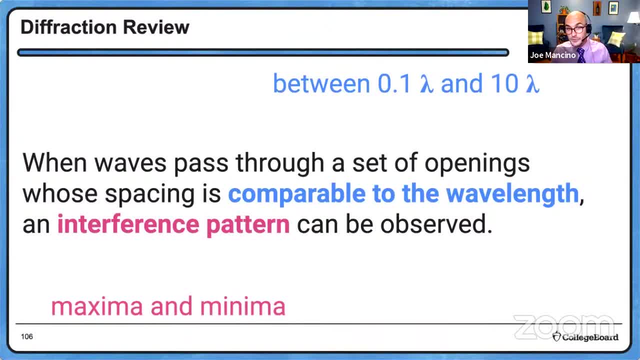 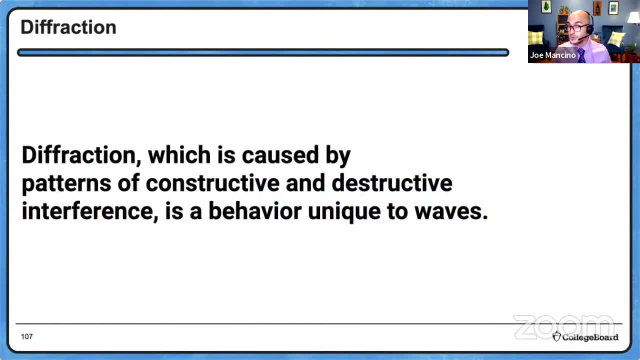 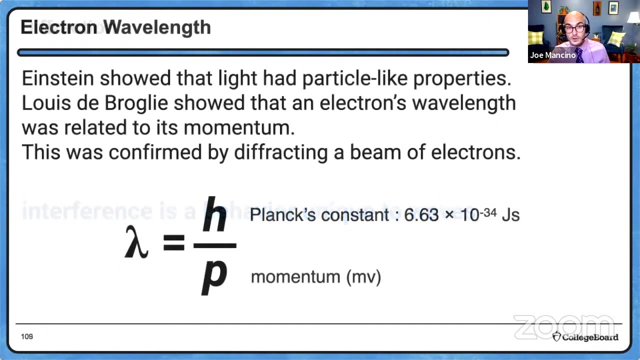 That's diffraction. Now, diffraction caused by constructive and destructive interference is a behavior unique to waves. Diffraction is something that waves do. It's interference, It's superposition, It is a very wave property. But if interference is a behavior unique to waves, then electrons shouldn't do it. 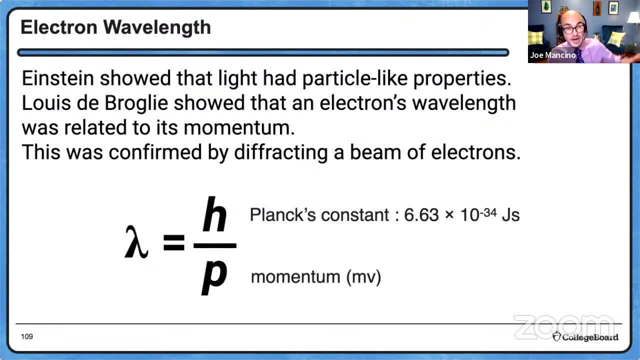 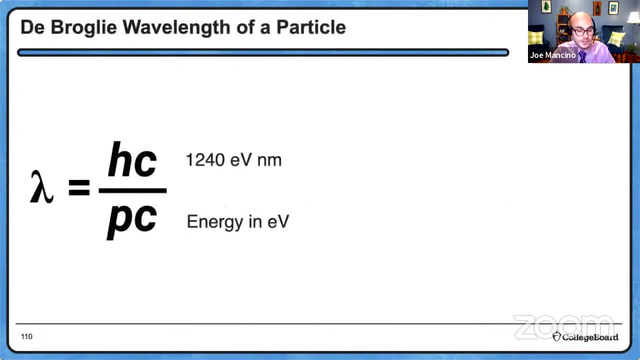 At the beginning of last century, Louis de Broglie hypothesized that electrons would do it. And don't worry about grabbing a screenshot of that equation, because here it is in three different contexts, three times. De Broglie hypothesized that the wavelength of an electron 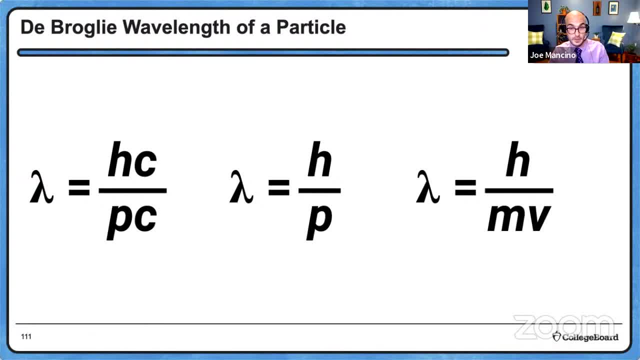 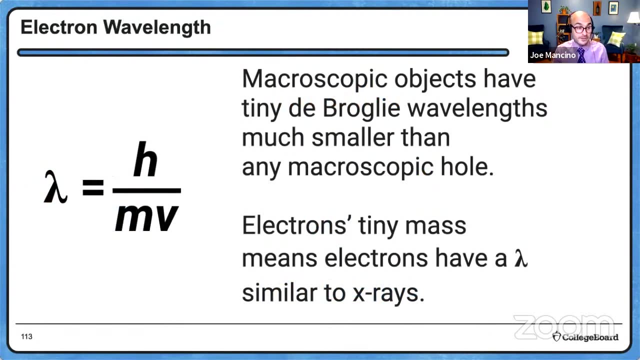 would be related to its momentum. But wait a minute. Wavelength is a wave-like property and momentum is a particle-like property, And that's okay. Electrons' tiny mass means that they have a wavelength. that's actually kind of similar to x-rays. 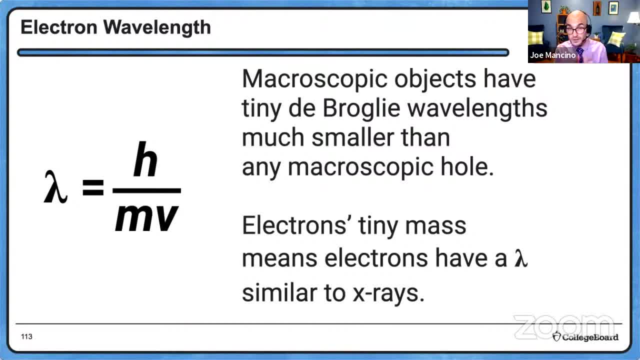 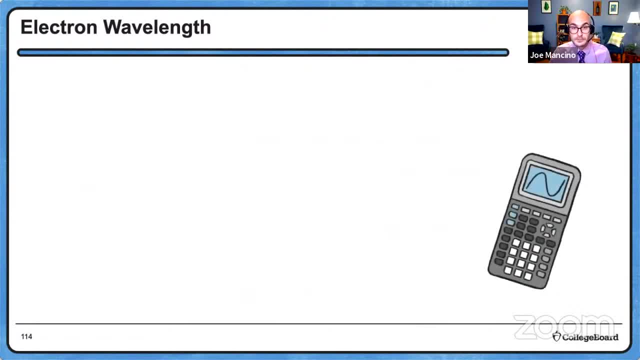 You and I have a wavelength that's way smaller than any doorway we could walk through, so we don't diffract. All right, This is question number one of your homework. It's something that you might have to do, So this is homework. 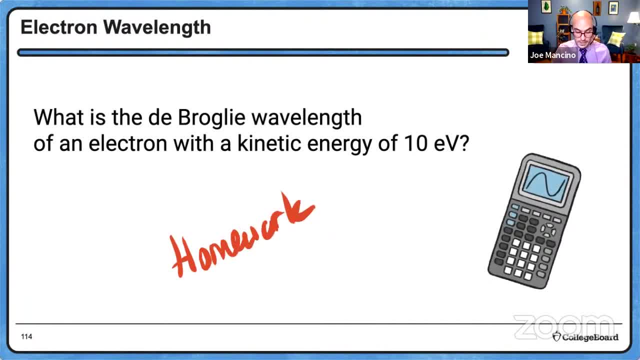 Mr Strautman will be talking to you about that one tomorrow. Can you calculate the de Broglie wavelength of an electron that has an energy of 10 electron volts? Here's hoping. Okay, the last thing that we have to talk about. 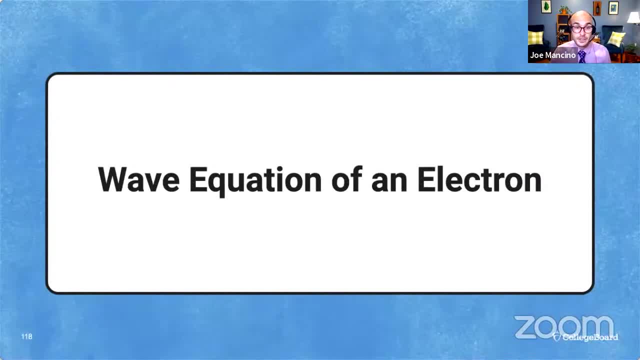 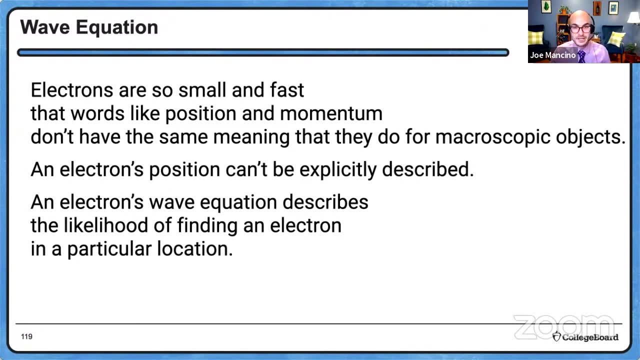 is the wave equation of an electron. See. electrons are so very small and fast that words like position and momentum, they don't have that much meaning as they do, as like for macroscopic objects. You and I have position, We have momentum. 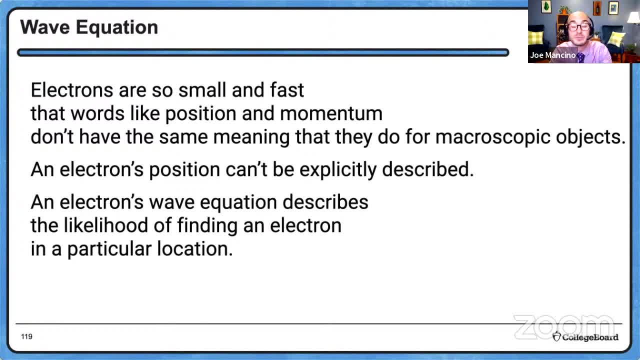 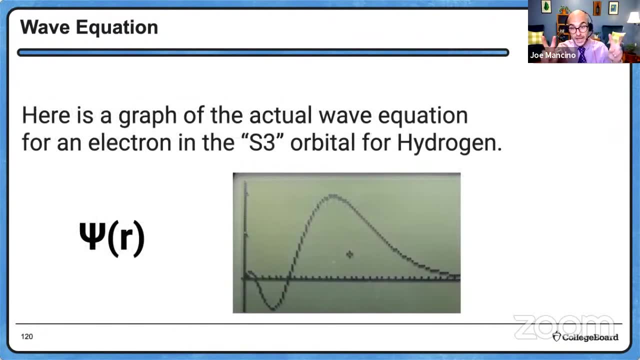 Electrons. their position can't be explicitly described. We have to describe electrons with a wave, An electron's wave equation. it's related to the likelihood of finding it somewhere. Now here actually is a graph of what's called the wave equation of the S3,. 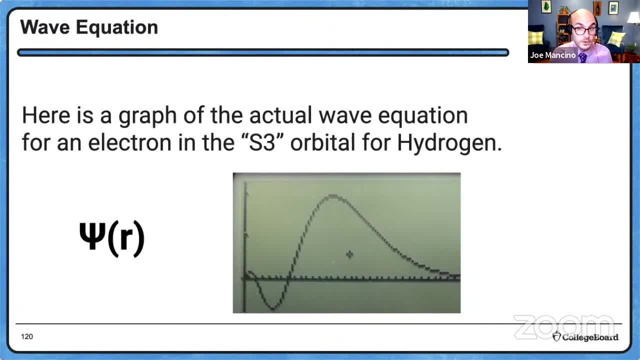 sorry for an electron in the S3 orbital for hydrogen. That doesn't tell you very much and I don't expect you to be able to interpret that. The important thing that you need to know is not strictly about the wave equation as a function of R. 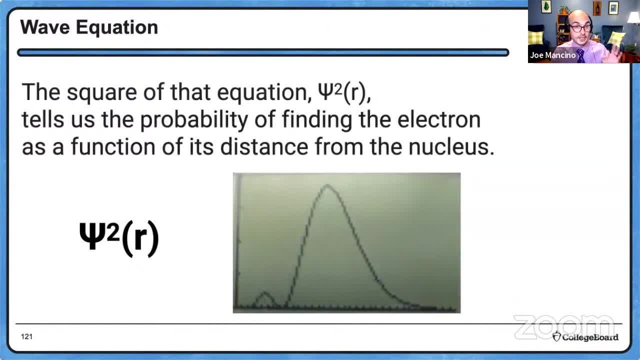 It's that this is really important: The square of the wave equation, psi squared. psi squared: When you square a wave equation, it tells you the likelihood of finding an electron somewhere. So if you're looking for an S3 electron, 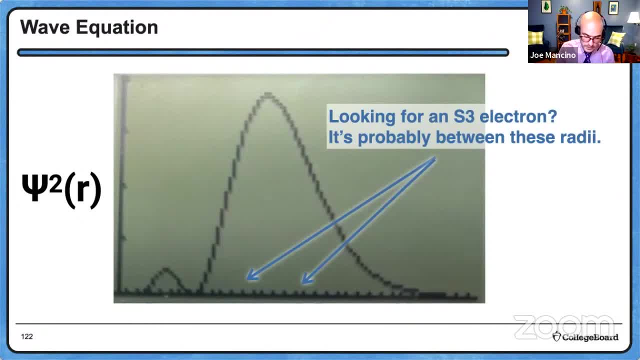 you're probably going to find it somewhere here. There's a pretty good likelihood that it's going to be around there. It's probably in there, But it's definitely not here. It's not there. It's not there. It's probably not going to be there. 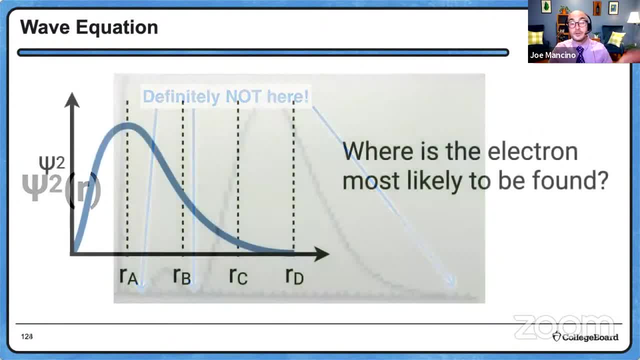 Okay, last couple questions for you. This one's easy. This is a graph of psi squared. Where would you be most likely to find this electron? Well, psi squared has a maximum at radius A. So yeah, radius A is where we'd be most likely to find this electron. 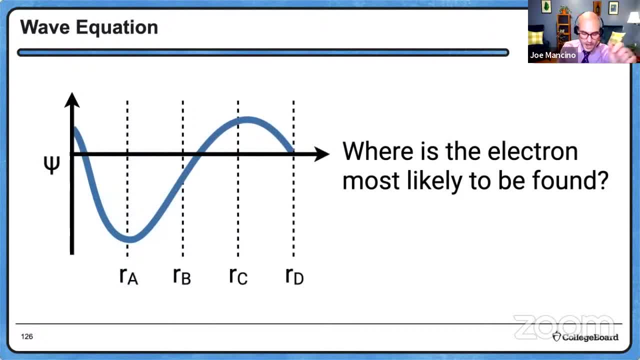 What about this electron? And note that the y-axis now is psi, not psi squared. You've got to think about psi squared there. Where would the square of this function be? Where would the square of this function be highest? Yeah, that's right. 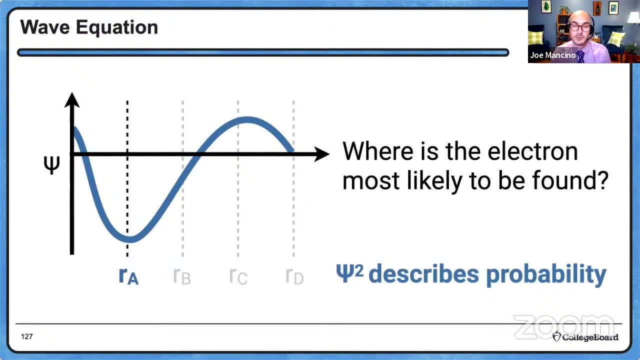 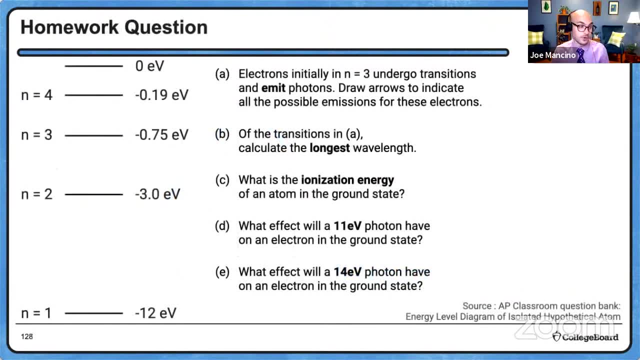 At point A. Psi squared defines probability. All right, So I said that was one of the two homework questions and I know I'm going over on your time here so I'll be quick. This is the other homework question. Please grab a screenshot of this. 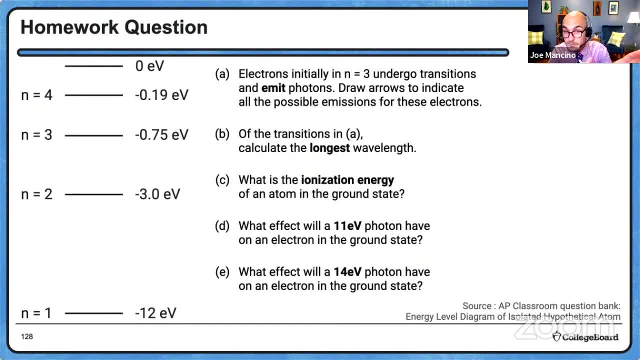 Mr Strautman will be opening with this tomorrow and reminding you how to calculate the wavelength of a 10 eV electron. Okay, Well, that was all of modern physics in 46 minutes. That was a lot of stuff. What should we take away? 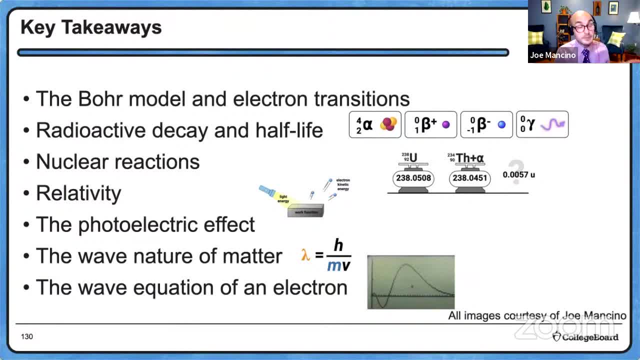 We need to know that the Bohr model is a pretty good model for what's going on with atoms. The Bohr model doesn't have the idea that electrons exist in these probability clouds, but it does explain electron transitions. You should know the four different radioactive particles. 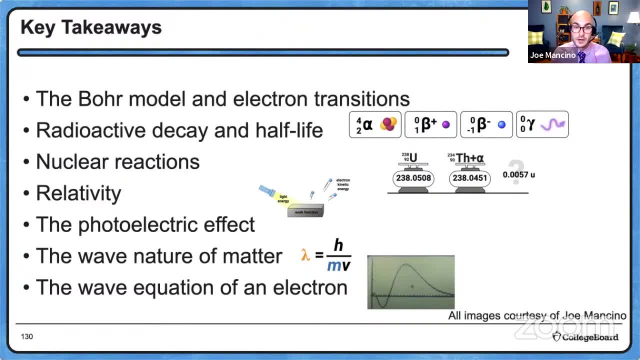 and the four different modes of radioactive decay that we talked about. You should also understand half-life. You should know that in a nuclear reaction total nucleon number is conserved and also charge is conserved. You should know that mass energy is conserved. 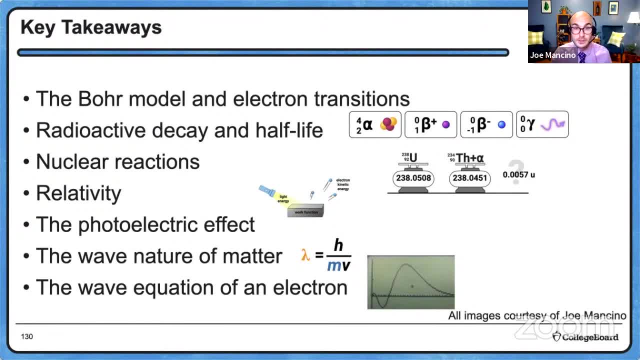 and how to calculate the amount of energy released. You should know that two observers, no matter how fast their relative motion is, they will always agree that the speed of light is 3 times 10 to the 8th meters per second. and they can disagree on everything else.